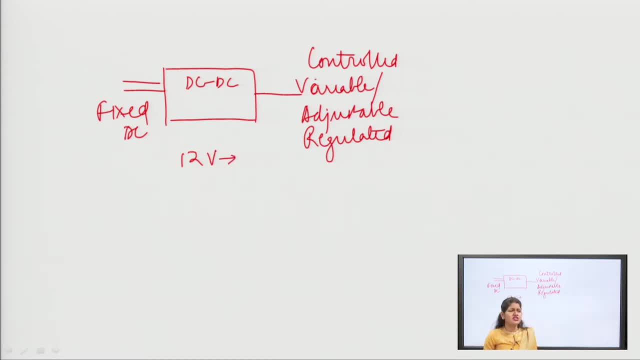 available in the lab, but there are some applications which require 5V, 6V, 3.3V voltages, like these. So in the lab we have this fixed 12V available, but our load, our application, is of 5V, 6V, 3.3V voltages, like these. 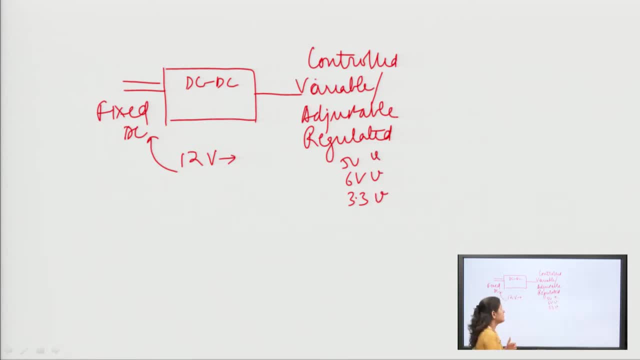 This is the application of DC voltages load. So in such cases, these DC to DC converters are used so that these 12 fixed volts can be stepped down or stepped up in any of these voltages Instead of 12,. this is the value of these voltages. 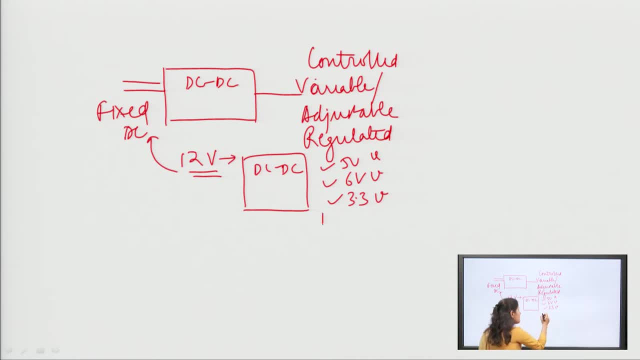 or this is the requirement of the load of these voltages. Apart from this, it may happen that we need 20V more than the fixed input DC, so every time we cannot change this fixed supply, Rather to get these voltages. we need this DC to DC. 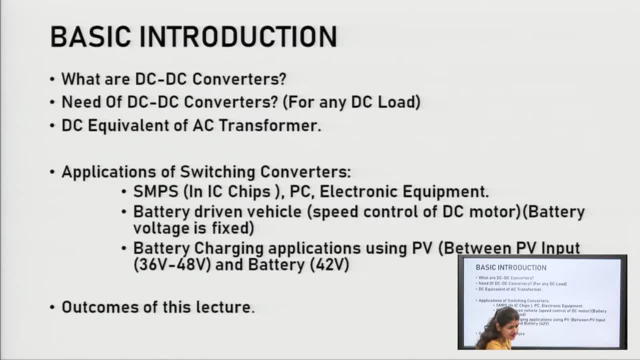 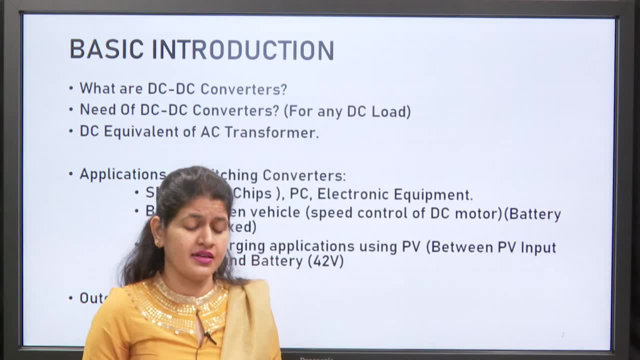 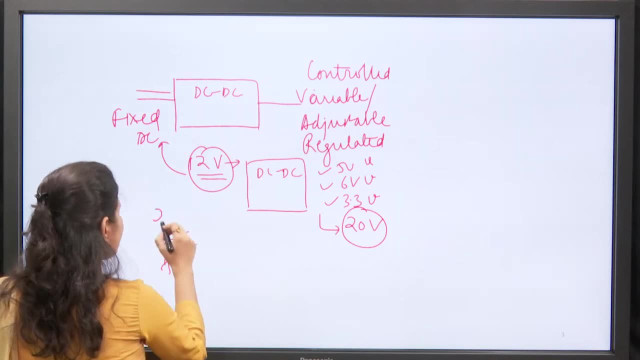 converter. Next, let us see one more thing: that DC to DC converters are also called DC equivalent of AC transformer. Why is this so? Because what does a transformer do? AC input voltage. let us assume any AC input voltage is 230V sin omega t. 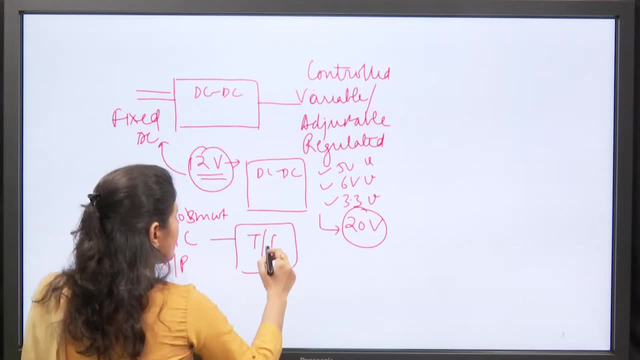 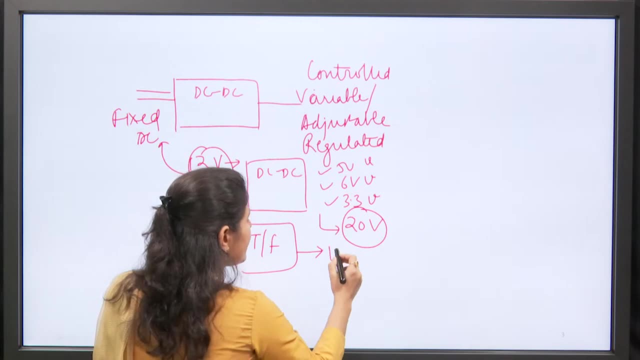 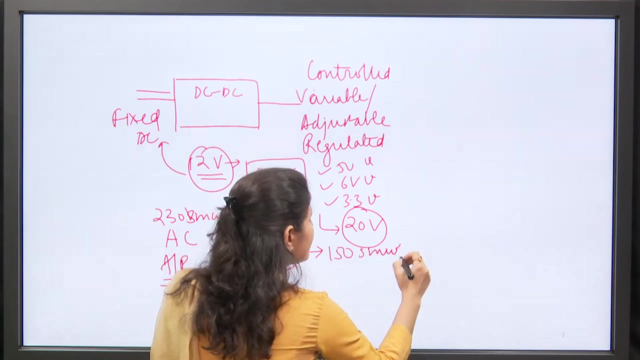 So what does a transformer do? A transformer steps up or steps down this voltage in any other voltage. Let us assume 230V sin omega t. So let us assume that 230V sin omega t will be converted into a step down transformer in 150 sin omega t and similarly, 230V sin omega t will be converted into a step up transformer. 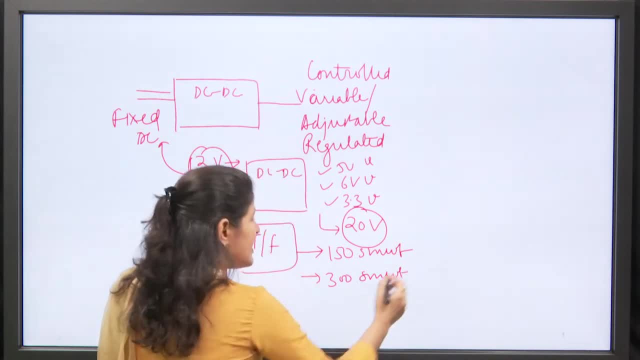 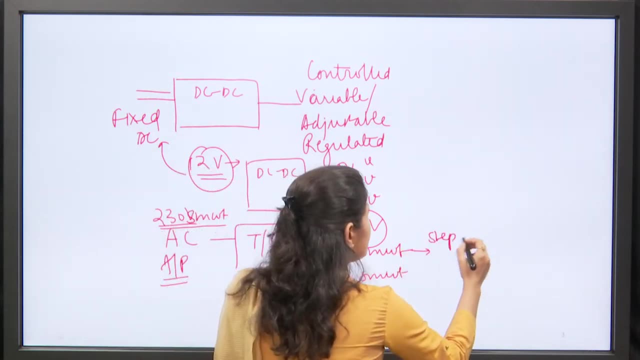 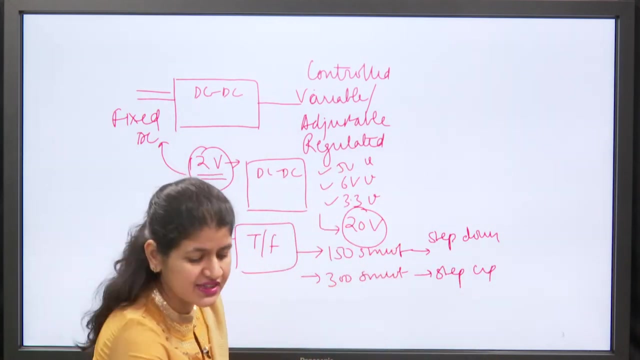 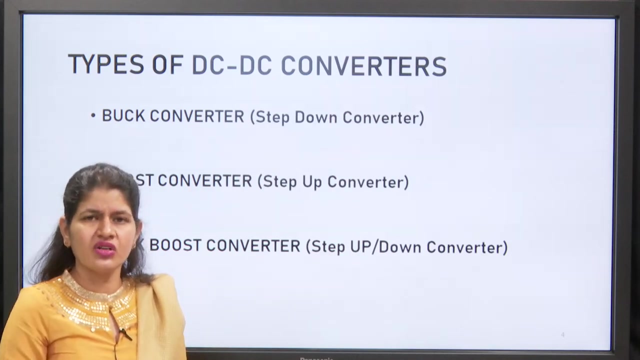 in 300 sin omega t. So, as we know, there are two types of AC to AC transformers. One is step down and the other is step up. So in this way we can convert DC to DC transformers. We can also classify DC to DC converters here. we will briefly know that which are the three step-up transformers, or step-down, or DC to DC converters available. 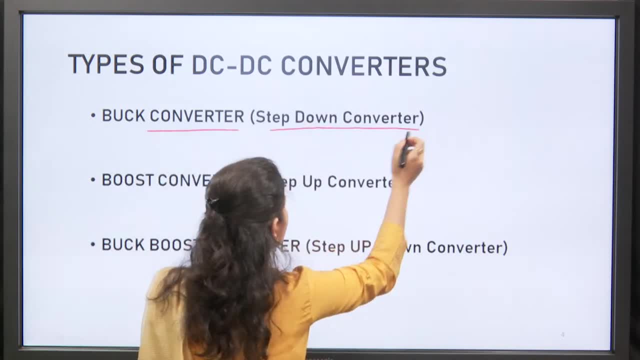 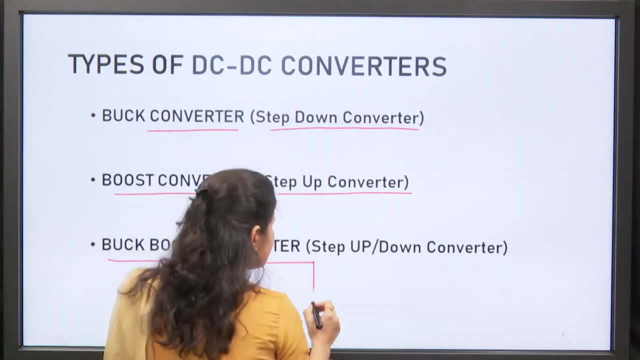 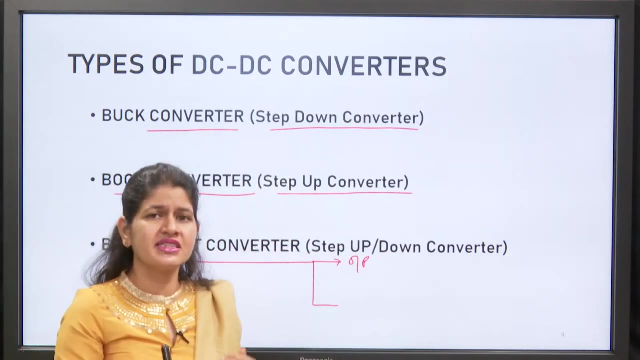 The first converter is buck converter, which we call as step-down converter. second is boost converter, which we call as step-up converter, and third is buck-boost converter. The speciality of this converter is that we can get both step-up and step-down voltage at the same output in the same converter. 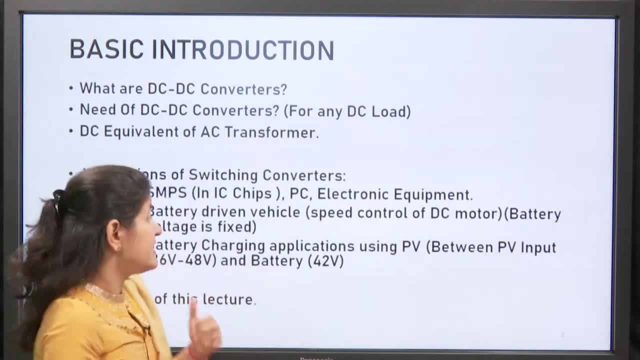 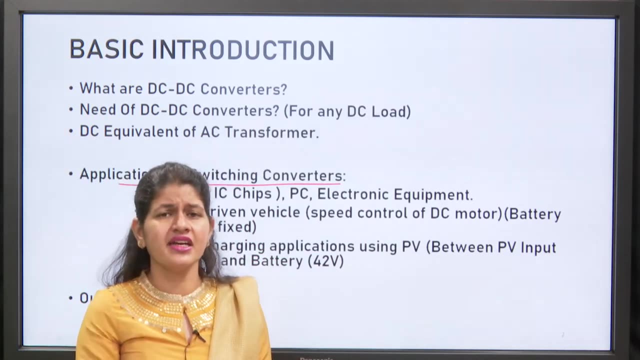 Next is its application. this is a very important part of it. What is its application? Switch to more power supply, SMPS- you have heard of SMPS. it is used in SMPS. All the PCs or any other electronic devices have small ICs in them. 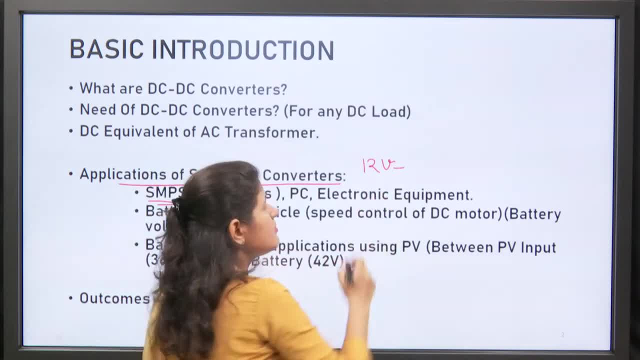 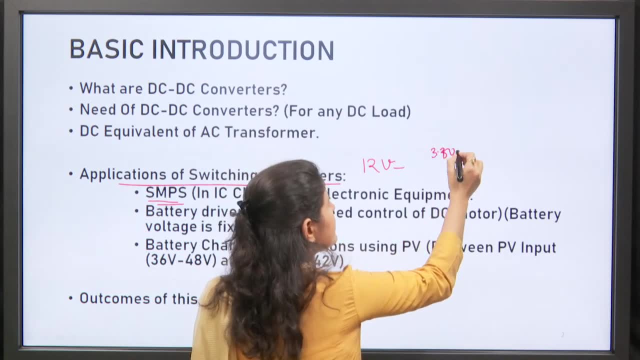 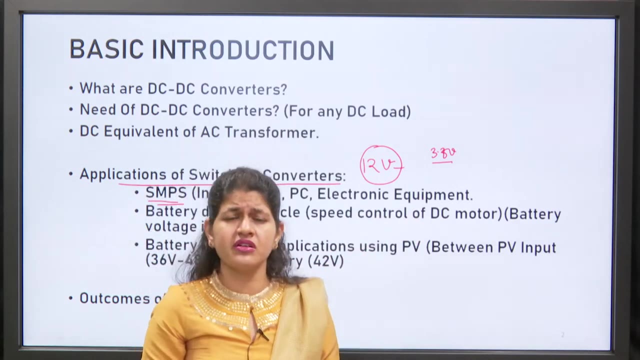 Let's assume there is 12 volts available, but there is a small IC in the PCs that require 3.3 volts. These 12 volts cannot be changed again and again, so in such applications we can use step-down converter. Next application is the battery driven vehicle. you must have seen that in many short distances we use battery driven vehicles. 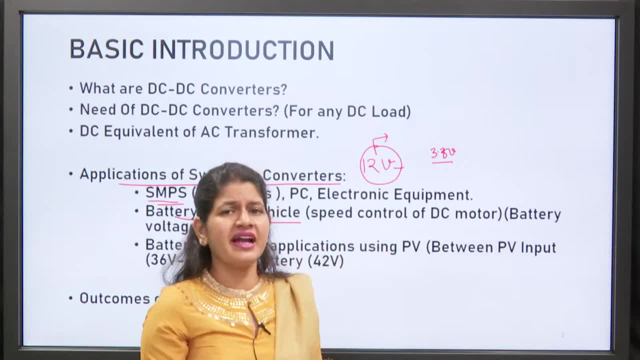 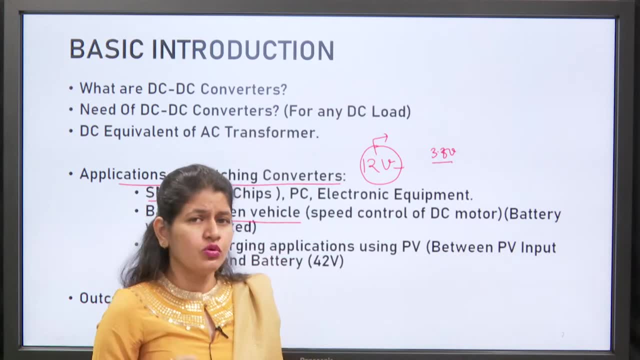 What happens in this also is that There is a fixed voltage in the battery but the motor, whose speed control we have to do it, needs different voltages because the speed is changing according to the voltage. So the varying voltage is given to us by the fixed DC or the fixed battery. 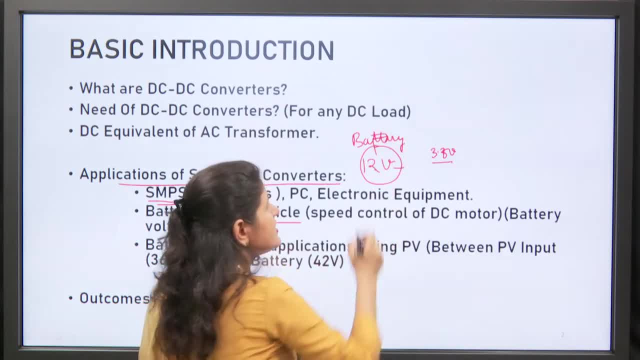 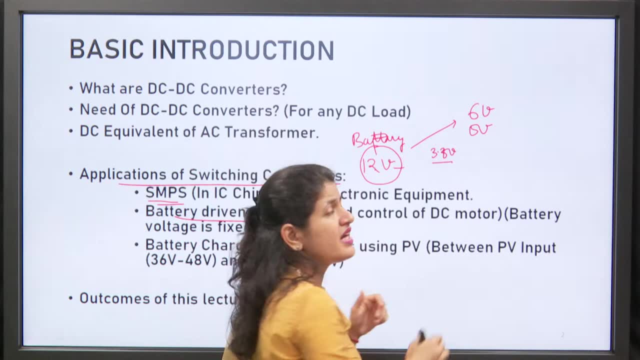 Let us assume that the 12 volt battery is in that electric vehicle and when we are doing speed control, sometimes it is 6 volt, sometimes it is 5 volt. so for this purpose also we can use these DC to DC converters. Another application is battery charging applications using PV. 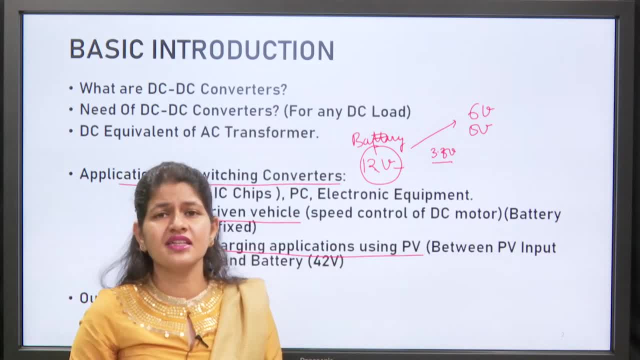 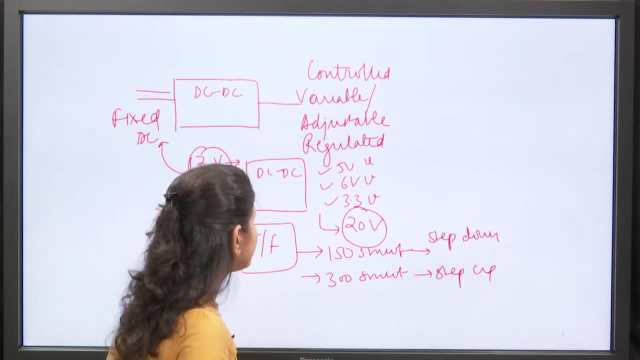 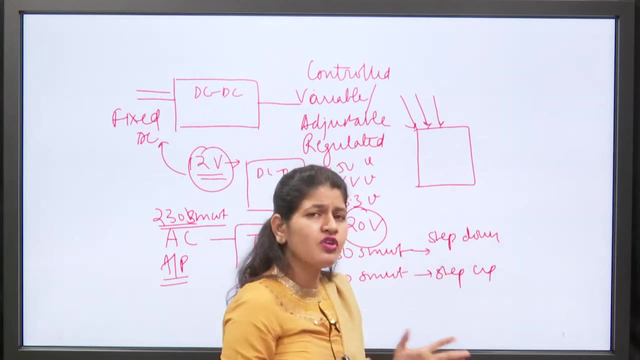 I have just told you that how much it is being used in PV industries or in solar industries or in renewable industries. So if we take an application of PV, what do we do in PV? Let us assume that there is a PV panel, the irradiation which is being applied on it, according to that, it changes its power. 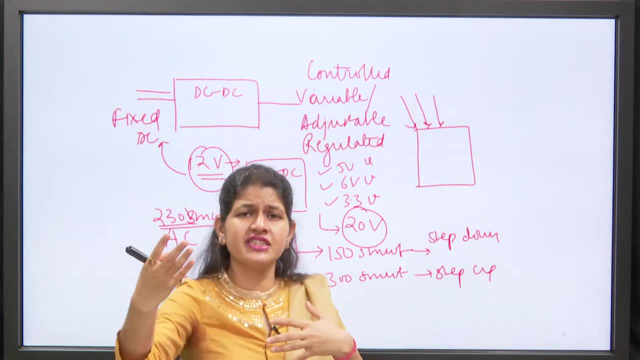 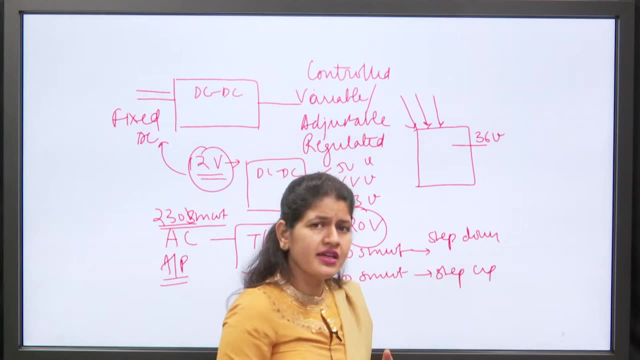 Sometimes some irradiation is being applied on it. Sometimes the sunlight is more, sometimes it is less. So on the basis of that, let us assume that this PV panel sometimes gives its output of 36 volts. sometimes the sunlight is more or it has changed so it started giving its output of 48 volts. 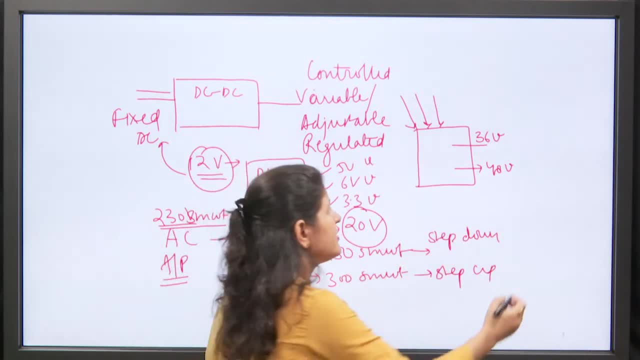 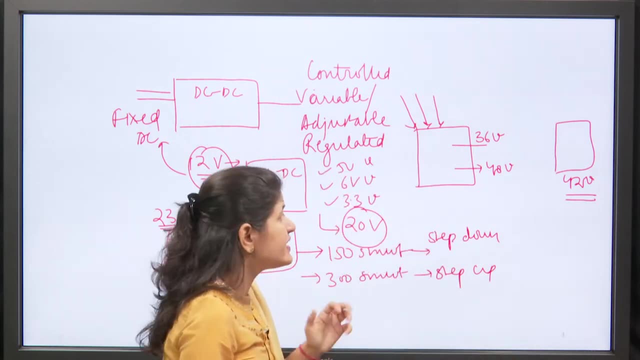 If we have to charge a battery from this PV panel and the fixed voltage of this battery is 42 volts- if we have to charge a battery of 42 volts- then what we will do for this We can use DC to DC converter. 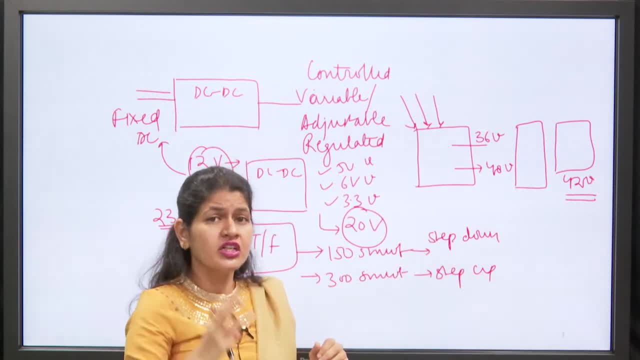 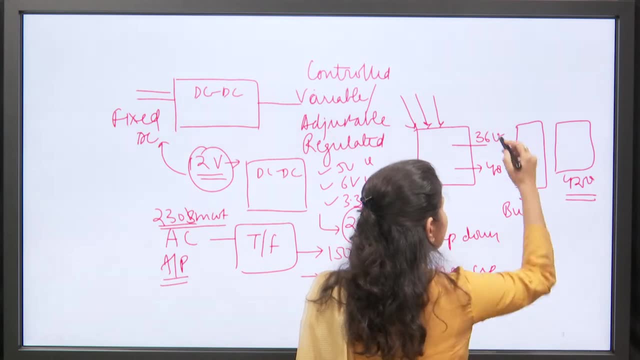 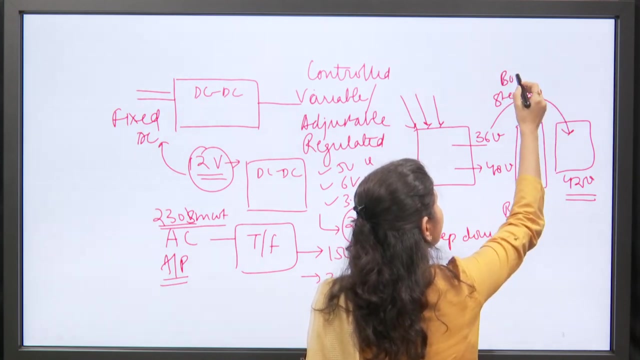 And which converter will be most appropriate here. The third type which we had studied: Bug boost converter. Bug boost converter. we can use here that when we want from 36 volts to 42 volts. that is, we want step up. If we want step up, then turn on its boost mode. 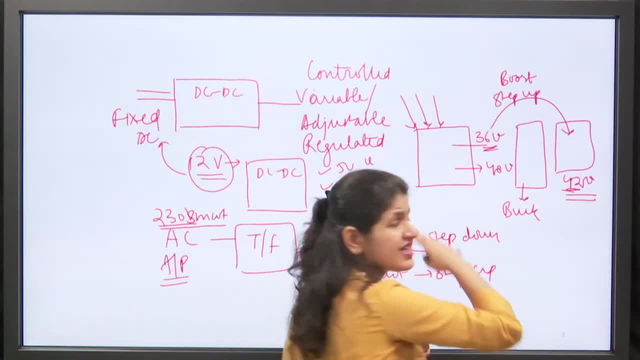 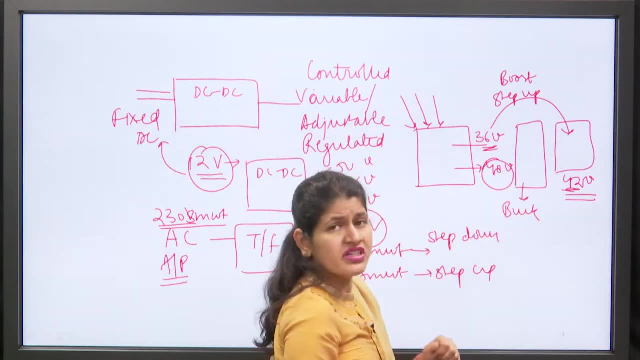 If we turn on the boost mode, then we will get step up voltage of 36 volts to 42 volts And similarly, whenever the solar panel is giving 48 volts and we have to charge a battery of 42 volts, then turn on its buck mode. 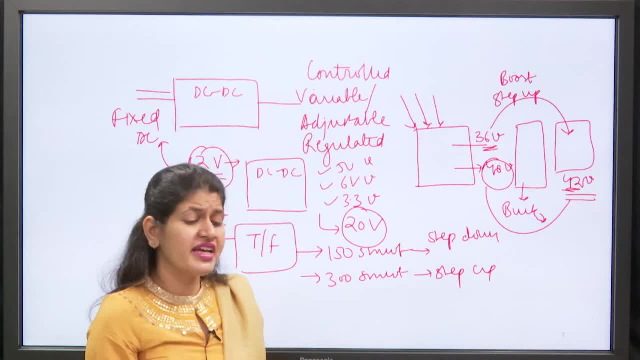 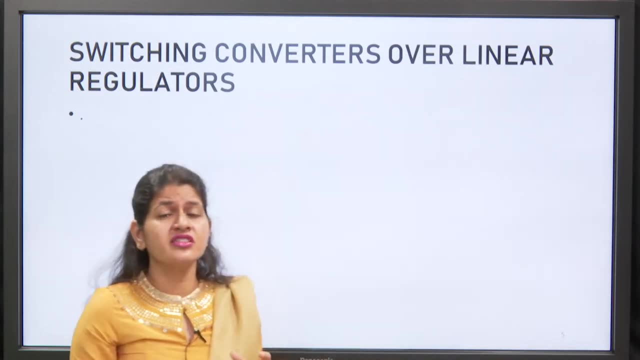 Buck mode means turn on the step down mode, So in PV applications we can use it a lot in this way. Next, let us come to what is the need of these buck boost converters? What is the need? What used to happen in the earlier times? 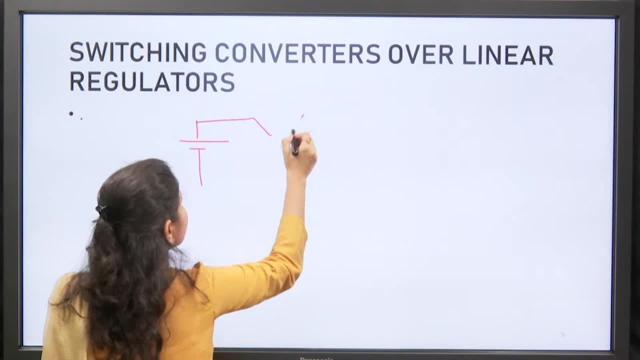 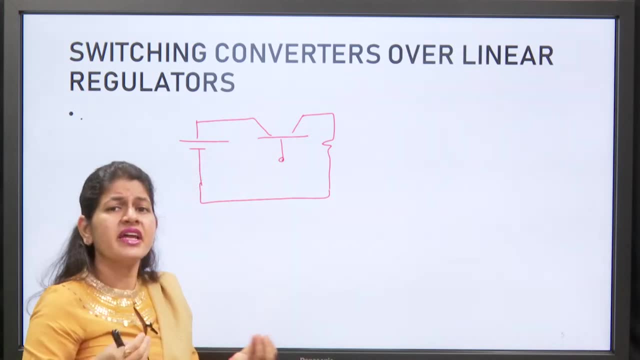 Earlier, what we used to use was linear regulators. What used to happen in linear regulators- This work which we are getting now, that we are getting step up voltage or we are getting step down voltage- we used to get this with the help of linear regulators. 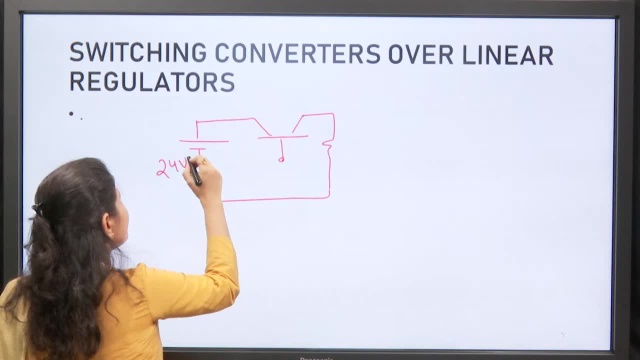 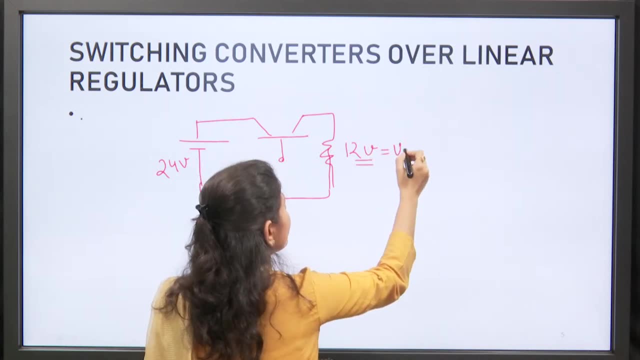 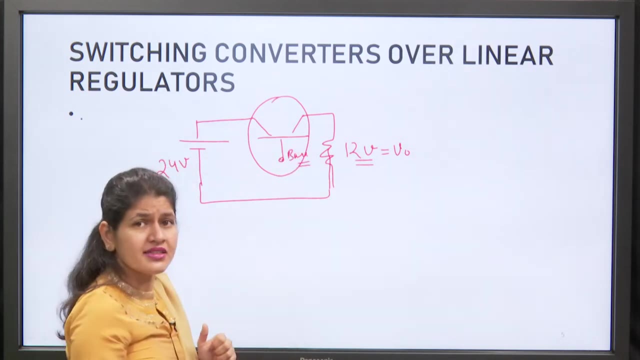 What do I mean by linear regulators? Let us assume that there is a 24-volt input supply here and we need 12-volt output on this load resistance. We need 12-volt output, So we used to control the base of this transistor in such a way. 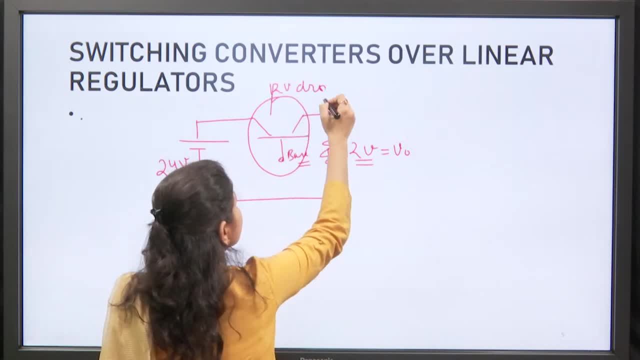 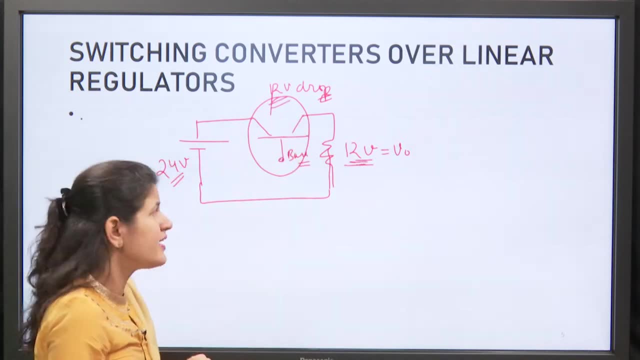 that we can get a drop of 12 volts across it. This is 24-volt input. If there is a drop of 12 volts here, then we can get 12 volts on V output. So in this way this transistor is working in a linear region. 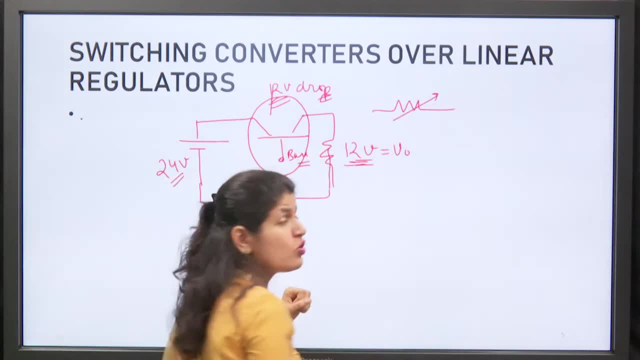 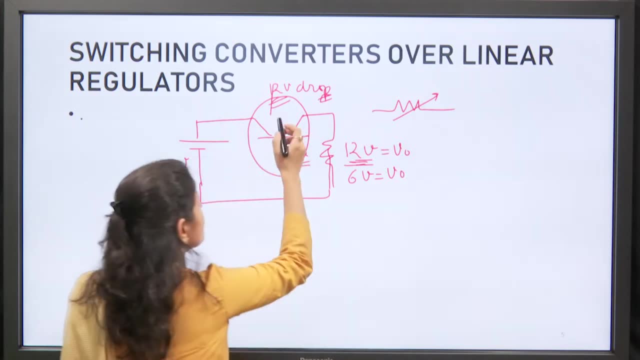 That is why we used to call it a linear resistor and that is why we call it a linear regulator. If, instead of 12 volts we need 6-volt output, we need 6-volt V output, then we can get a drop of 18 volts here. 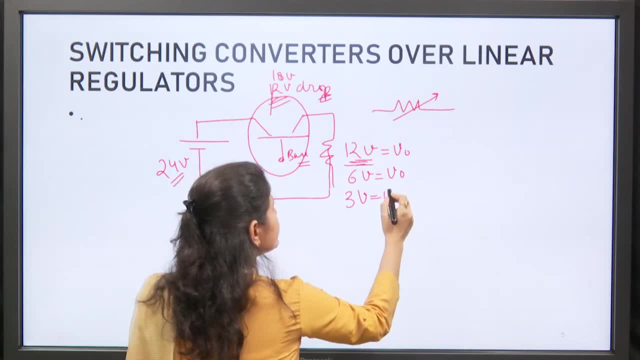 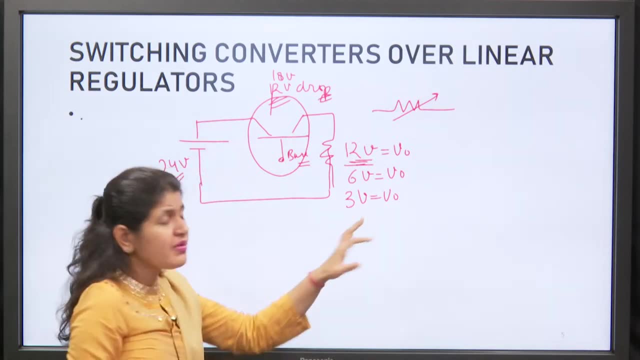 In the same way, if we need 3-volt V output, then we can get a further voltage drop here so that we can get the desired V output. So we could achieve this step-up and step-down in the same way. 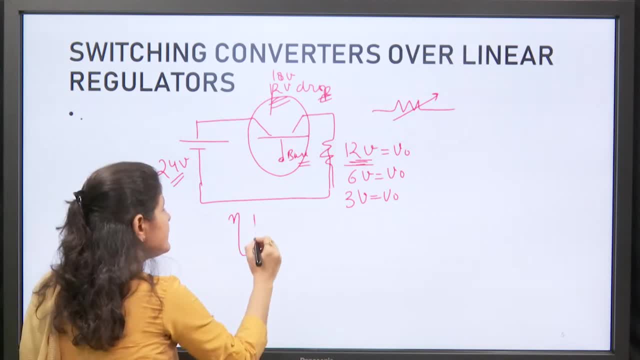 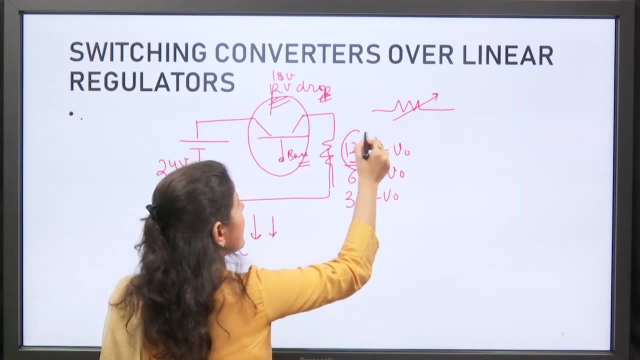 But what was the problem in this? The problem was efficiency. Efficiency is greatly reduced. How is it reduced If we are getting 12 volts here? and if there is a drop of 12 volts here, then the power available on the output. 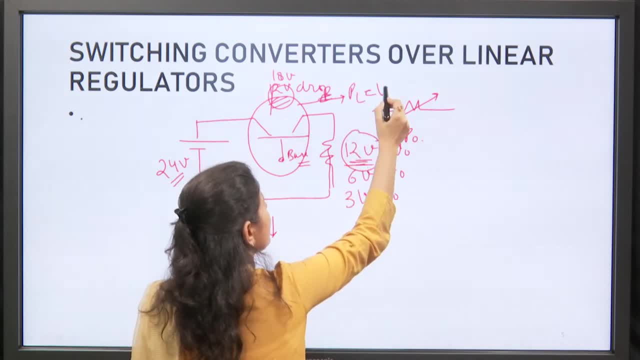 that is also the power loss here, because power is equal to V into I. So if we are getting 12 volts here, then this is also the power loss. If we are getting 6 volts here and if there is a drop of 18 volts here. 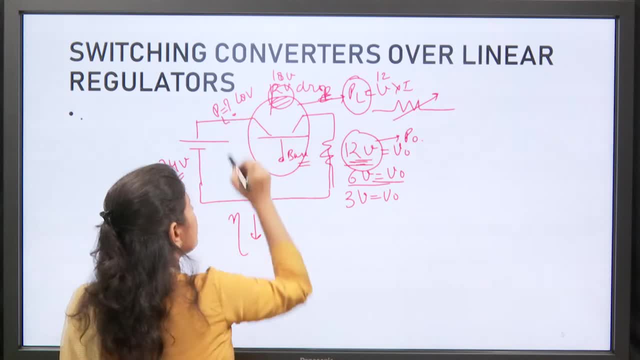 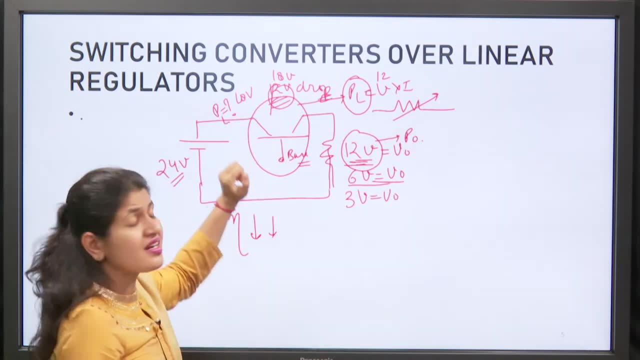 then the power loss. here this PL power loss is even more. According to 6 volts, we are getting power here: P is equal to V into I, And according to 18 volts, P is equal to V into I. This much drop is happening here. 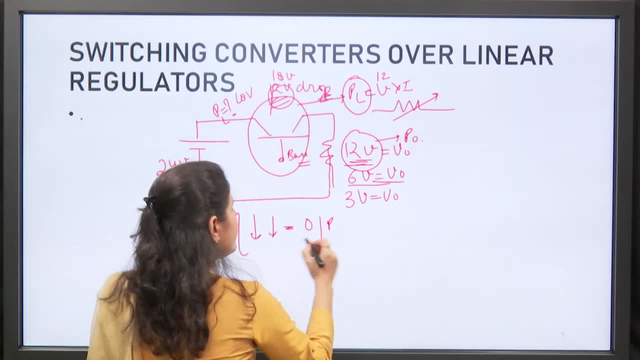 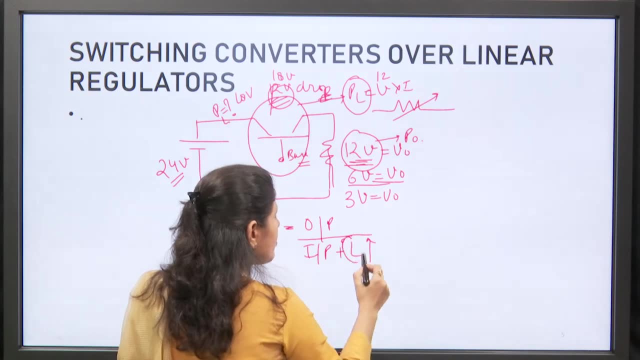 So what is efficiency? So what is efficiency Output upon input plus losses? So if losses keep increasing this much, or PL, the power loss, if it keeps increasing this much, then efficiency will keep decreasing. This is its drawback. 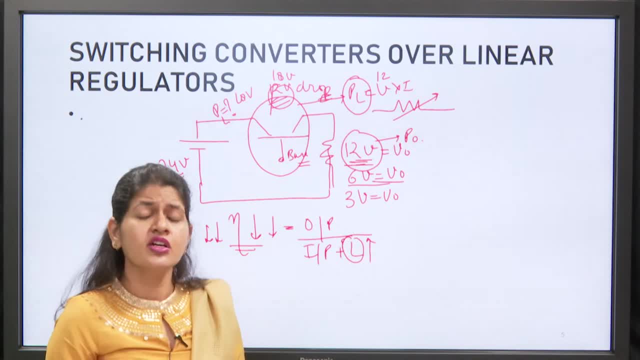 due to which we needed to use switching regulator. So what else do we do in switching regulator? This is the power loss problem. So instead of this, we use a switch. How is that switch? Let's see in this slide. 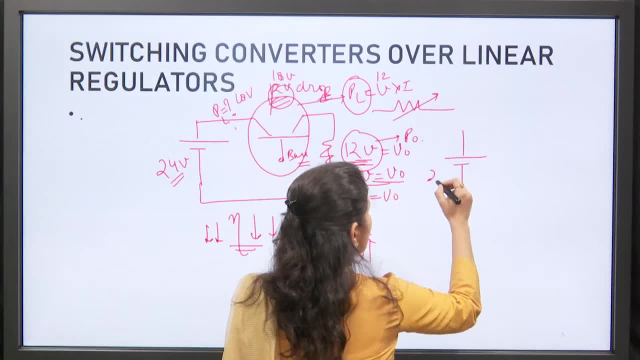 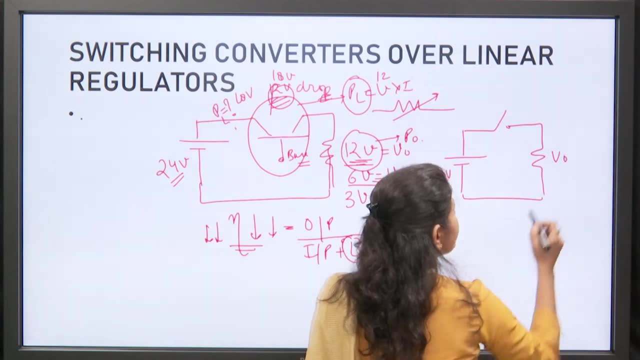 Let's see in this slide: How is this switch? Let's assume that here there is 24 volts DC, So we used a switch here And this is the load output, whatever output we need. So how will this switch work? 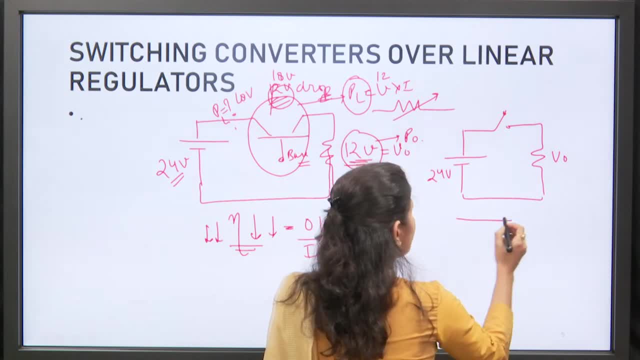 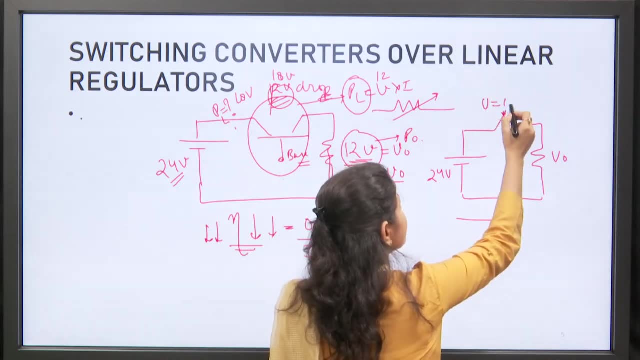 Once on or once off. So when this switch is working in on mode- let's assume that this switch is on- then this short circuit will behave like a wire. So how much voltage drop will there be across this? It will be zero. 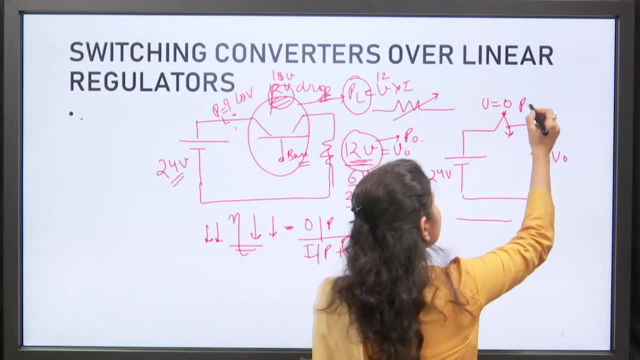 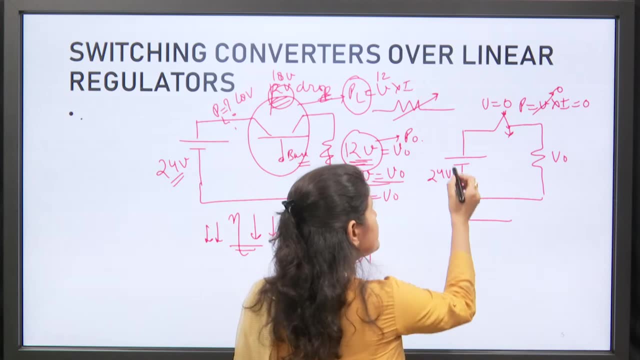 because the voltage of short circuit is zero. So what will happen? P is equal to V into I. If this part is zero, then this power will also be zero. Okay, So the input voltage will be the same as the V output. 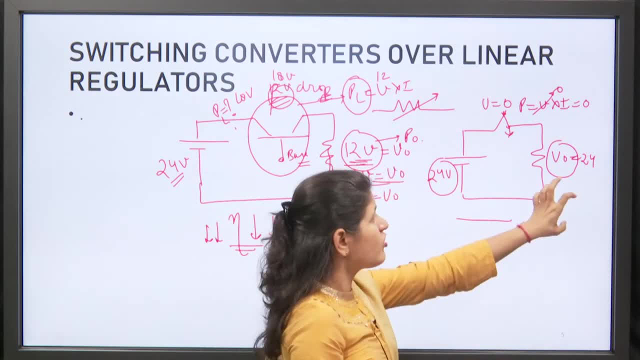 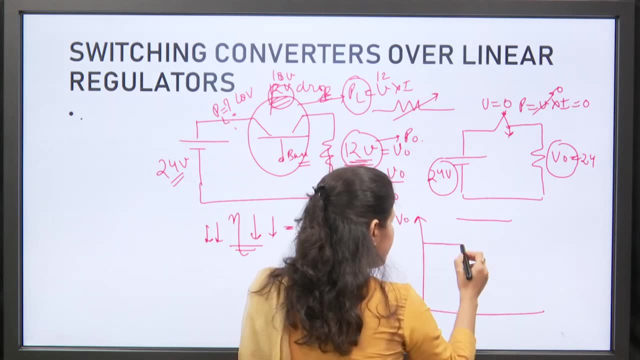 Right, Because it is short, so it is parallel. So V output will be equal to V input. So see how will we get the output, This V output, when we switched on ie when T was on. 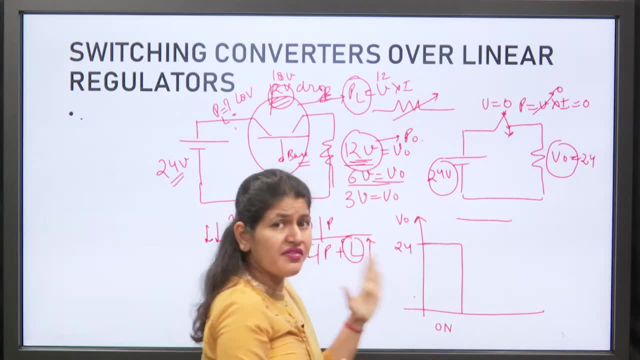 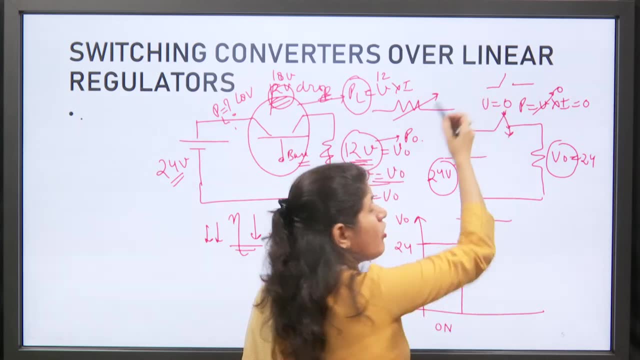 we got the complete V output, ie 24, the complete V input. Now see when the switch is on. when the switch is on like this: when the switch is on, so what does on mean? The wire is open. 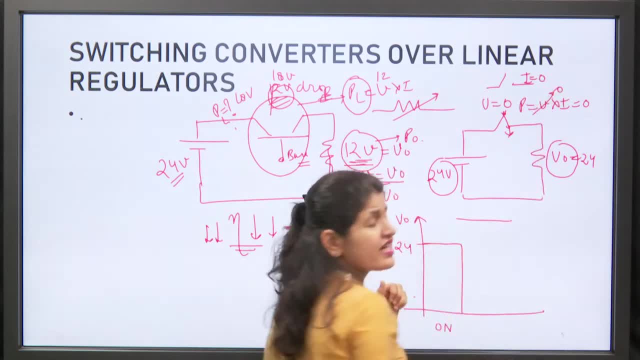 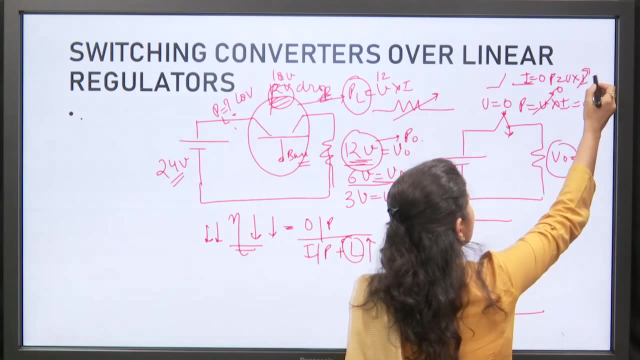 Okay. So how much will be the value of i? across this, No current will be able to flow. i will be zero. So P is equal to V into I. if the i part is zero, then also the power will be zero. 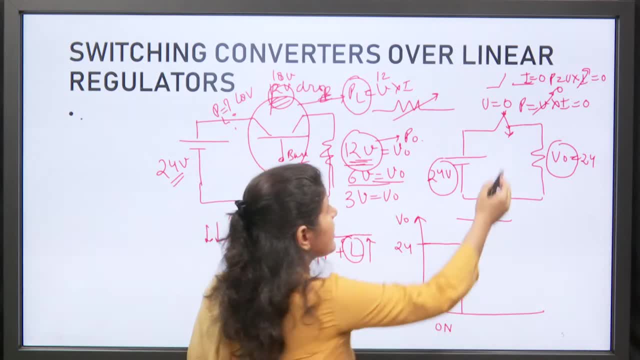 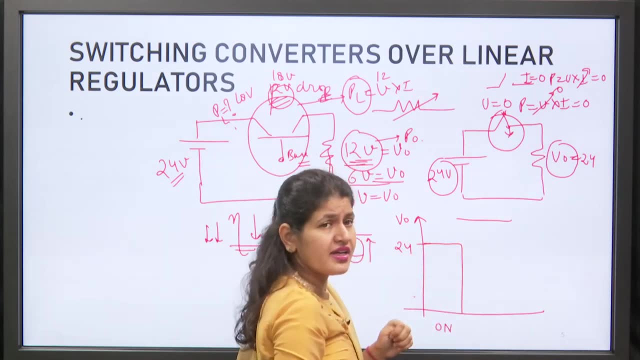 Okay, So when the switch is on, then also the power loss across this is zero. But how much output will we get? If this switch is on, then no current will be able to flow from here to here. So how much output will we get? 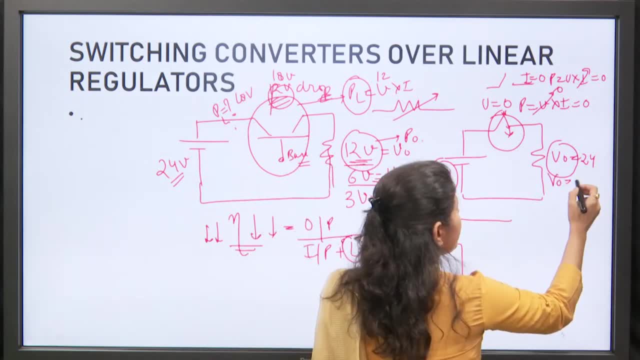 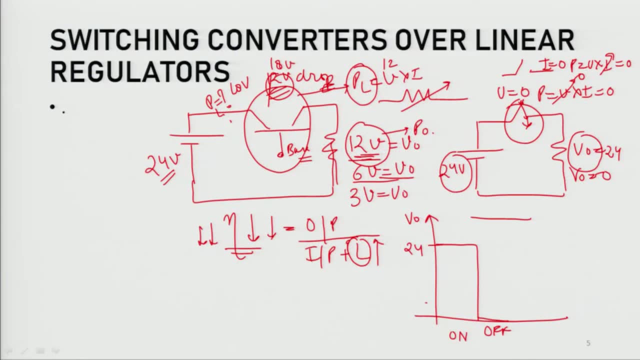 Zero. Okay, In the case of on, we will get the output as zero. So see, we got the output as zero. Okay, ie the switch is off. Off means when the switch is open and on means when the switch is conducting. 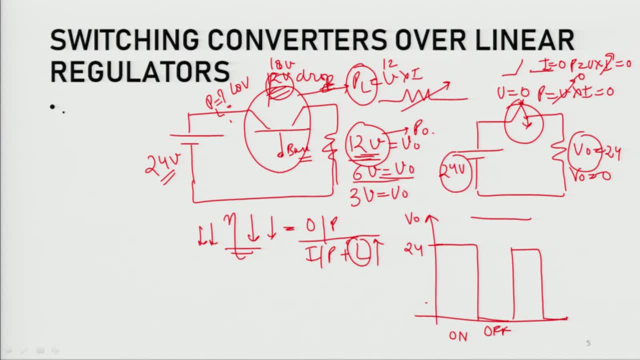 Okay, So in this way we will get the voltage on off, on off in this way. Now, if we take its average, then how much will it be? It will be 12 volts. Okay, So now we are getting 12 volts. 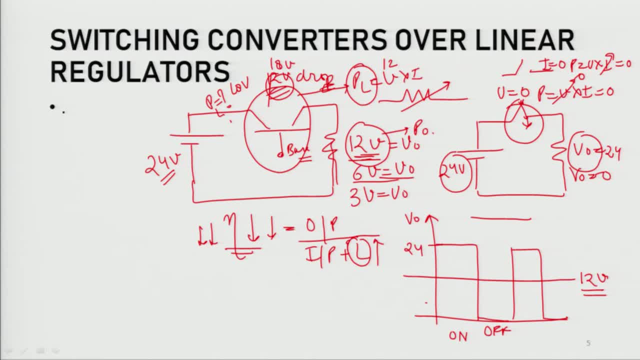 at the output without any loss, without any power loss. So these types of converters, we call them switching converters. So these types of converters, we call them switching converters. Okay, Let's make it clean here. These types of converters. 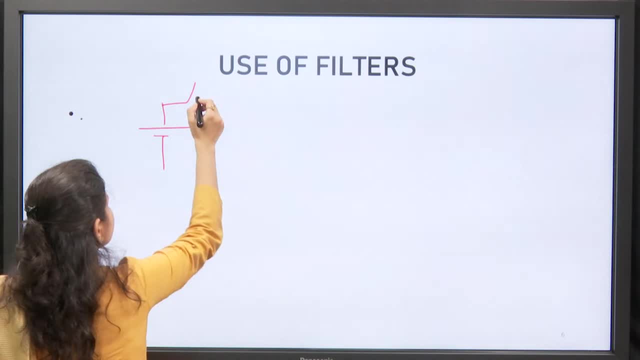 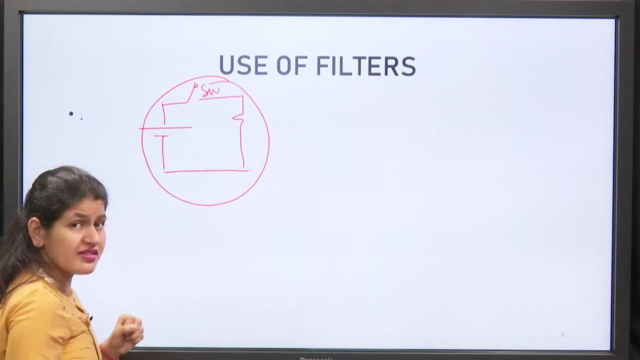 this is the input source, this is the switch, and here is the resistance. Okay, This is the switch. These types of converters- we call them switching converters. And how, with what name, did we get to know them? We called them choppers. 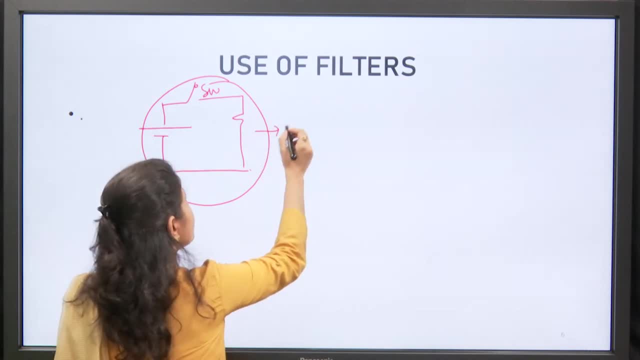 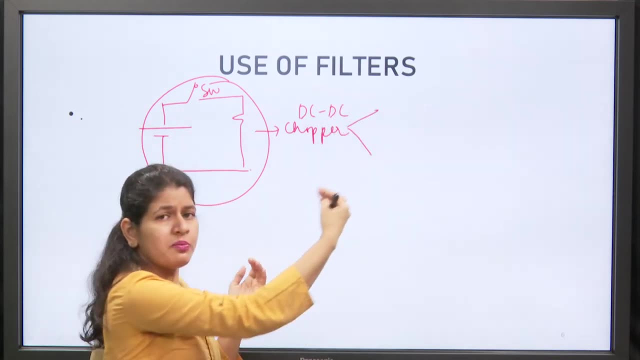 Okay, Choppers. Choppers are also the same DC to DC converters. There were choppers too. Step up chopper, step down chopper. two choppers were available, like this. But now, what is the drawback in this? 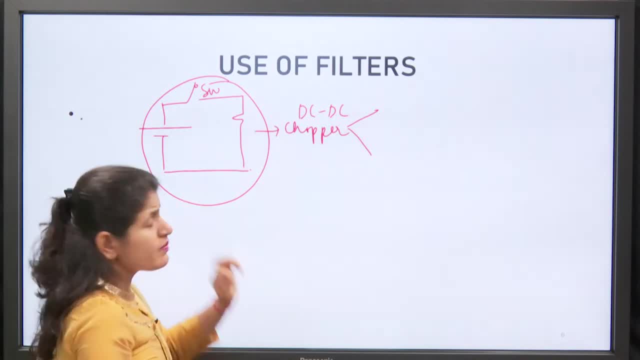 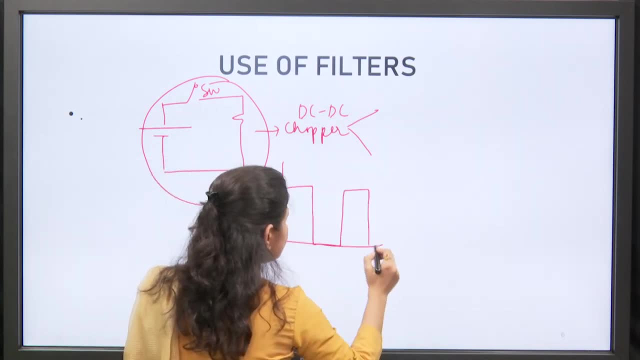 The drawback of this is that the chopper is a DC to DC converter, So the drawback of this is that the output we are getting is like this: Okay, The output we are getting is like this: Okay, This is the V output. 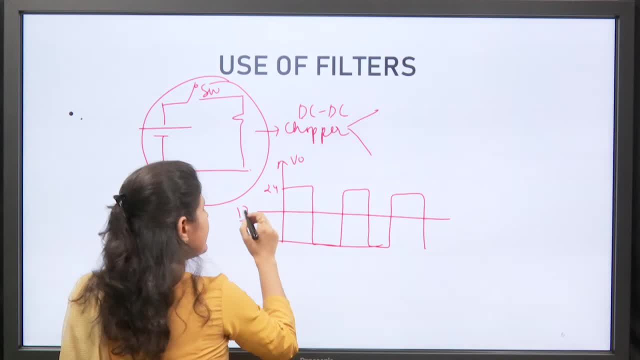 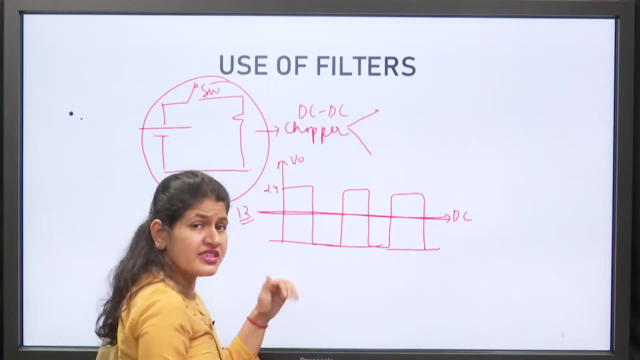 and this was 24 and this was 12.. Okay, This is the V output. This is the desired value. This is the average value. This is the DC value that we need, But apart from that, we are also getting some AC sinusoidal components. 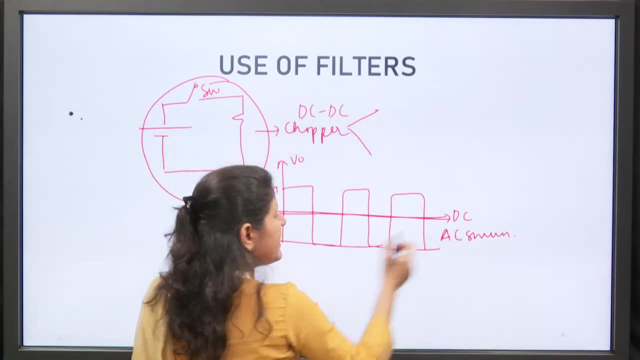 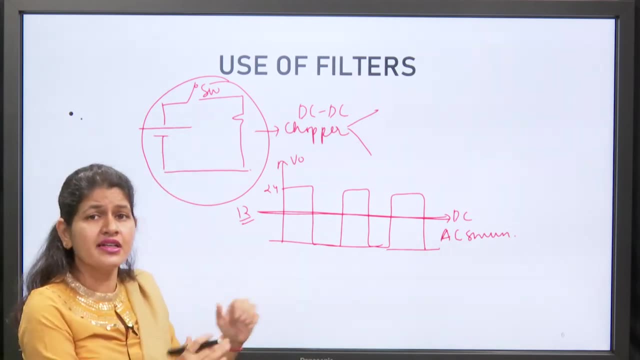 Because of this we are not getting plain DC. So to remove these AC components, we have to remove these components and in the same circuit, we will apply a filter. Which filter will we apply? This is DC. This is the switch. 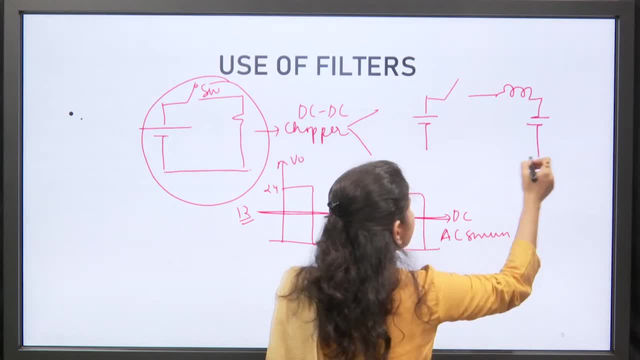 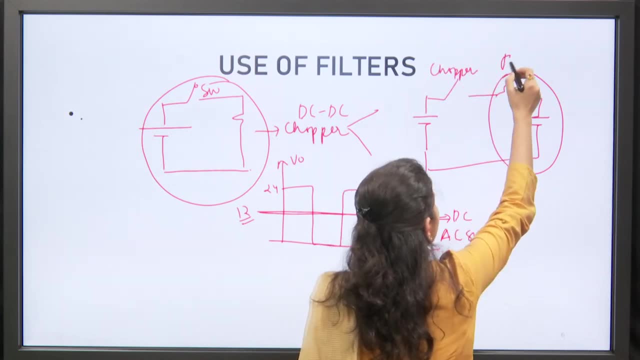 And here an L and a C, Which is a low pass filter, Which means in this chopper circuit- this part was a chopper- and in this chopper circuit, if we apply a filter and after that here is the load resistance. 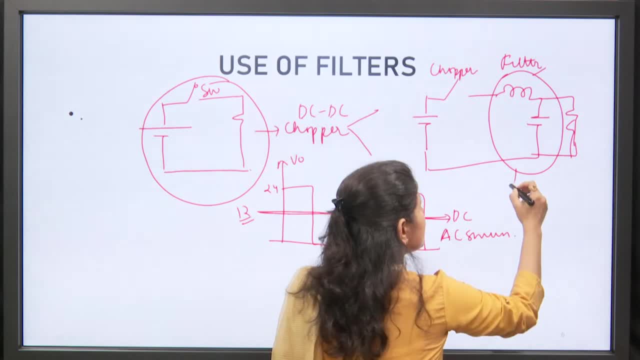 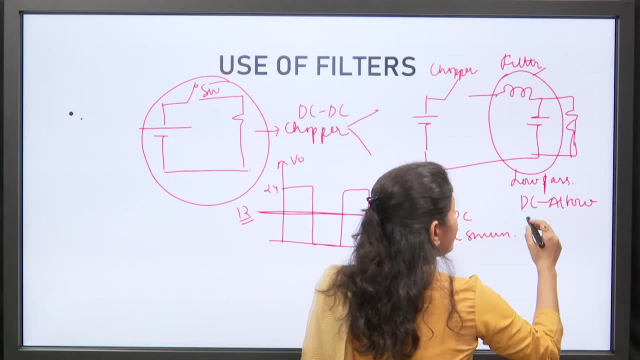 This is the load resistance. If we apply a filter, then the filter is a low pass filter. Right LC filter is a low pass filter which allows DC in the output and blocks AC components in the output. So, with the help of this, 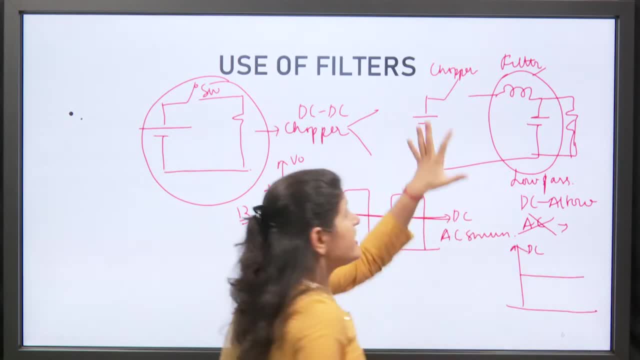 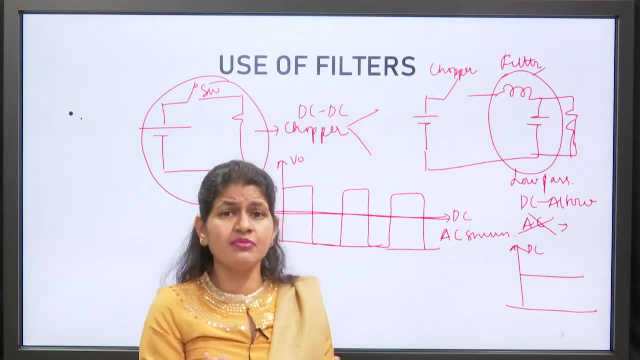 we can get a plain DC Right. So if we apply a LC filter in the chopper, if we apply a LC filter in the step up chopper, then it will become a boost converter. It will be easy to remember by name. 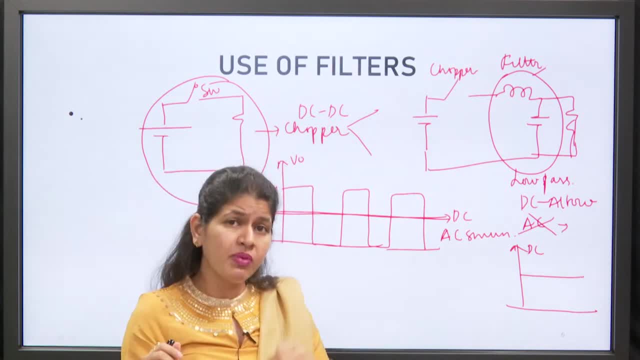 Boost means we are getting something big. If we apply a LC filter in the step down chopper, then it will become a buck converter. It will also step down. So in the buck converter there is a difference in the buck boost and buck. 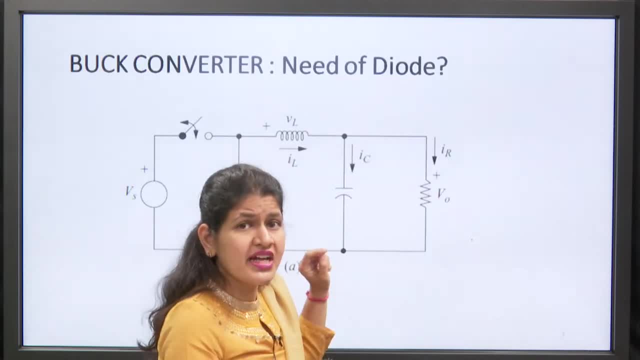 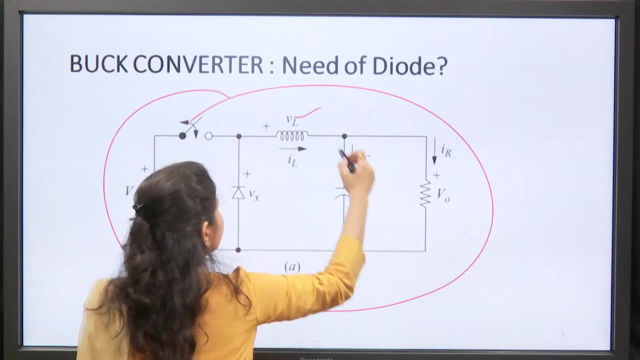 boost converter that an additional LC filter is applied Right Now. let us know one more thing here that what is the need of diode. This is the complete circuit of buck converter, So you can see that there is L filter, C filter. 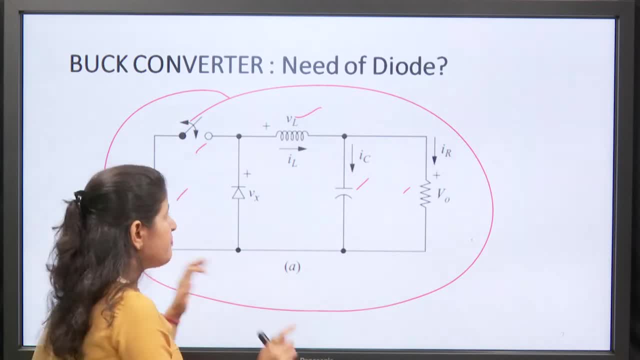 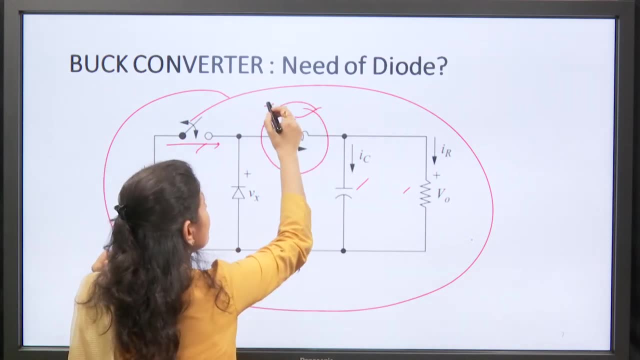 R switch. this is it, But there is a diode also applied here. What is the requirement of this diode? In the first half, this inductor has energized itself. If this diode is not applied here, then this inductor. 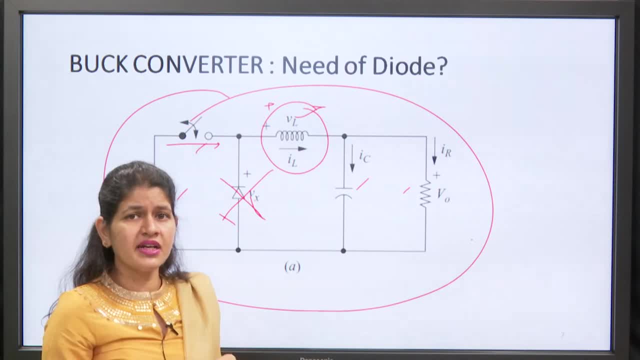 will not get any path to be de-energized, and if the inductor will store so much energy inside it, then it will cause sparking problem, which is disadvantageous. So for this case we use a diode of this polarity, which helps. 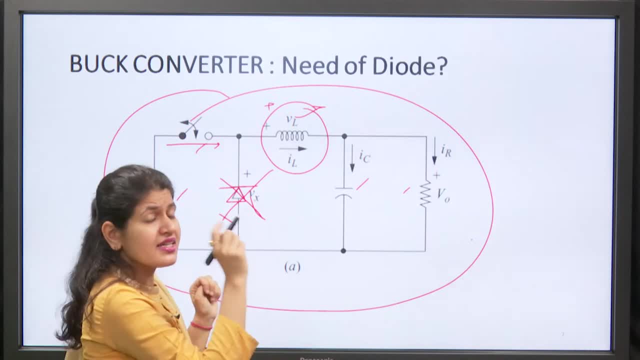 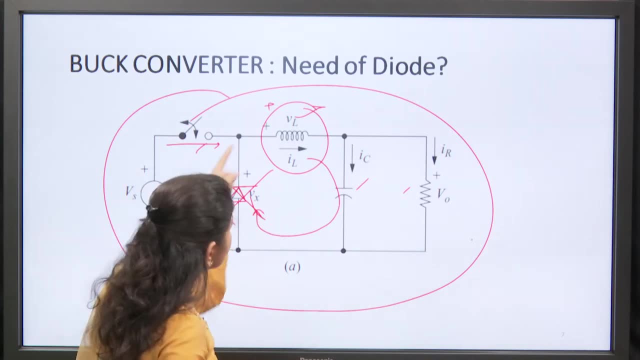 the inductor to be de-energized. That means when we open the switch, the inductor will be energized. So the inductor will be energized and the current which is stored inside it will be released. So this is the use. 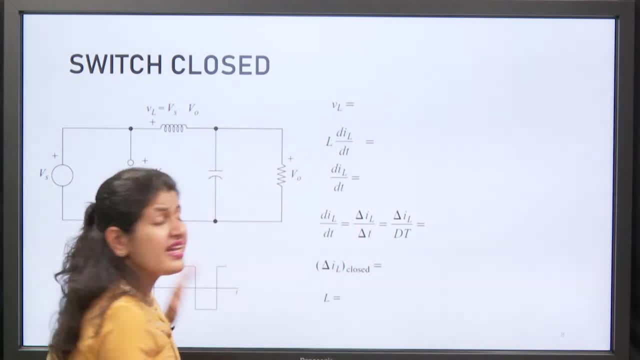 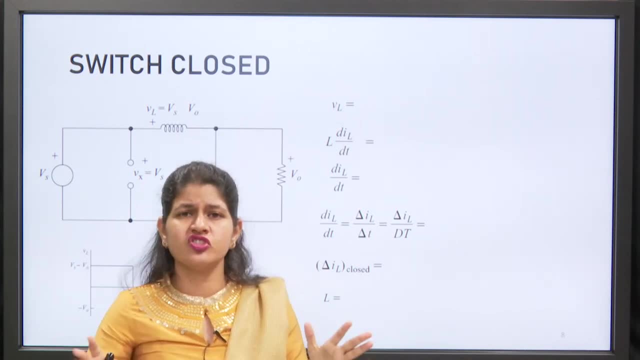 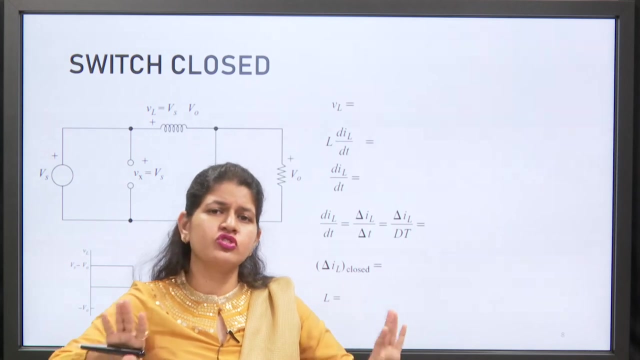 of diode which is applied in the buck converter circuit. Now let's see the analysis part. First, let's know why we are studying analysis. We study analysis because in any industry there is an application that 100V is available and 50V. 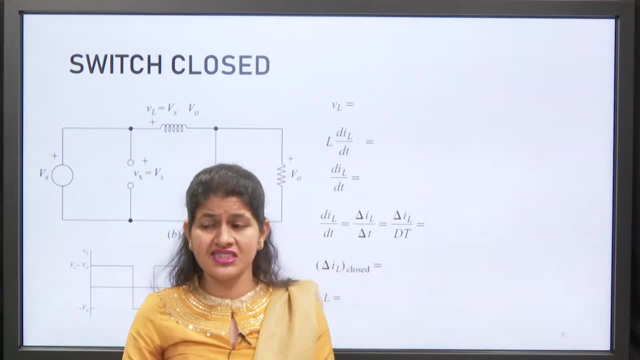 is the load, That means the fixed supply for which you have been hired as a power engineer in the industry, wants you to make a 50V converter because we have 100V available, So we need a buck converter. So any converter. 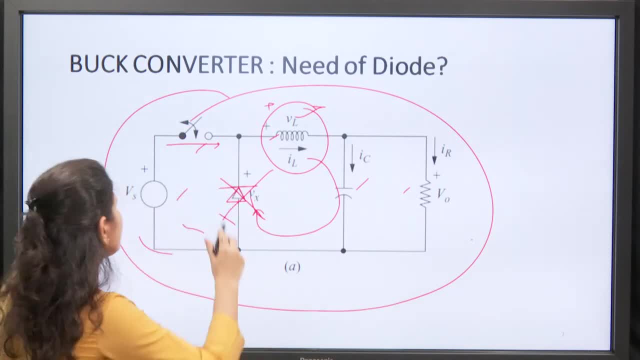 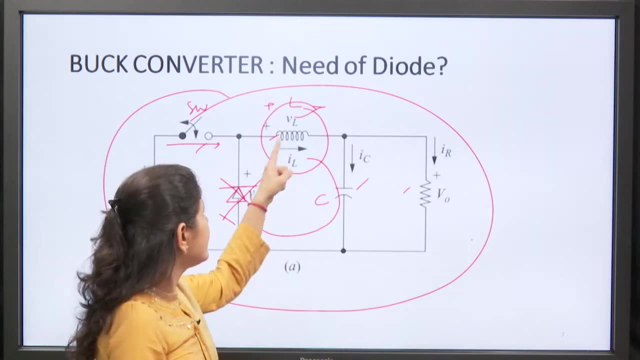 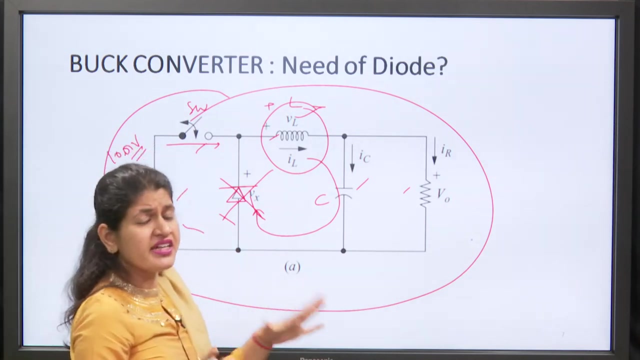 you can see, but any converter will have these elements. There will be a switch, an inductor and a capacitor. So until you know that this inductor and capacitor is 100V input, that means fixed supply is available in the company or in the industry. 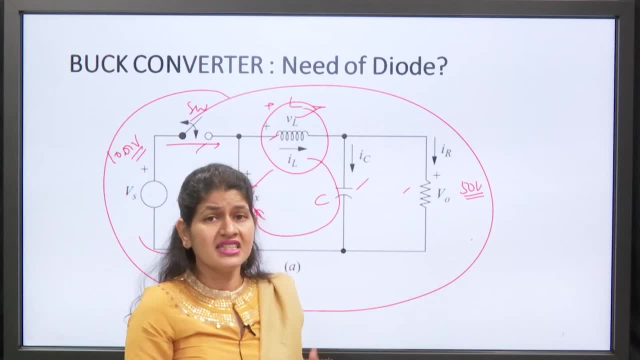 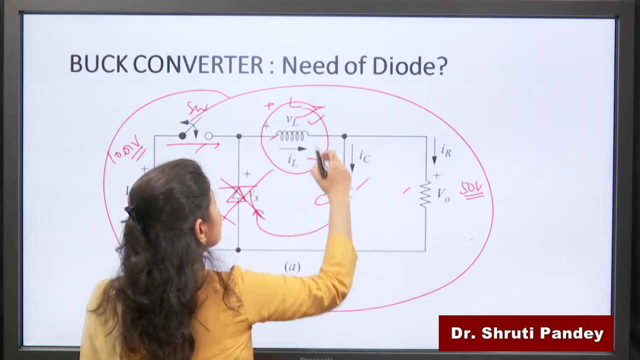 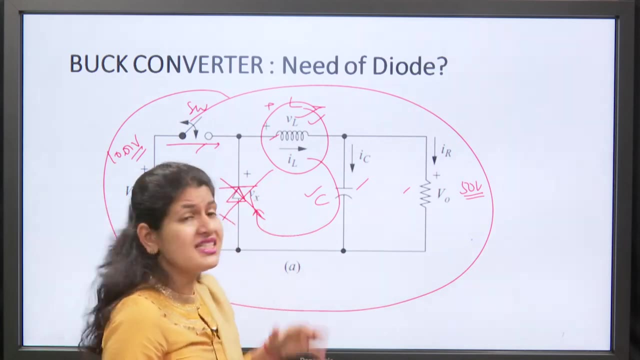 and we have an application of 50V output or 50V load for which we have to design this buck converter. You know this, but until you know the value of L and C, you cannot make an appropriate buck converter, because L and C are big in themselves. 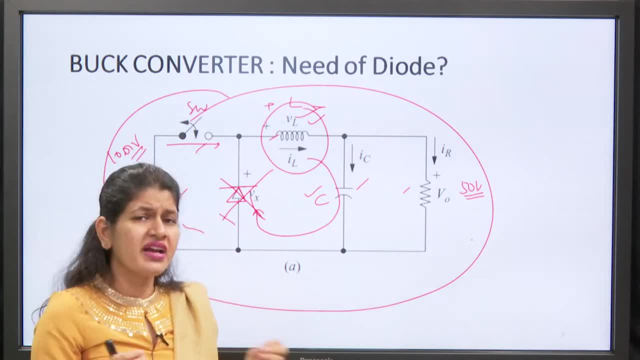 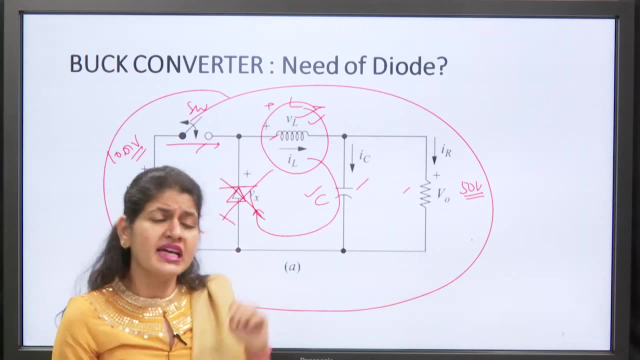 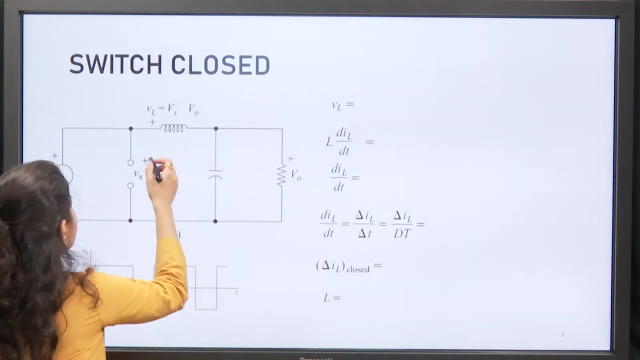 If you take any random value of L, then you cannot take anything randomly. To make an efficient converter, it is important to know the appropriate value of L and C. That is why we do analysis of all the converters. So let's start with close switch. 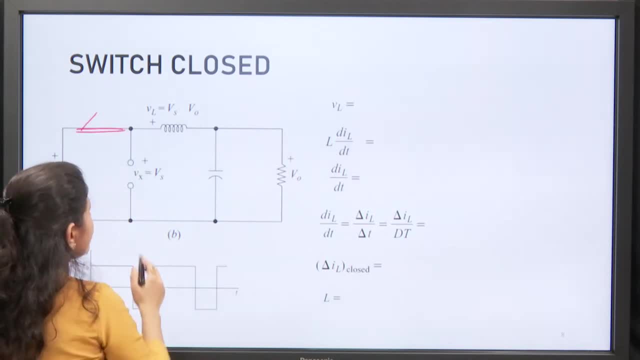 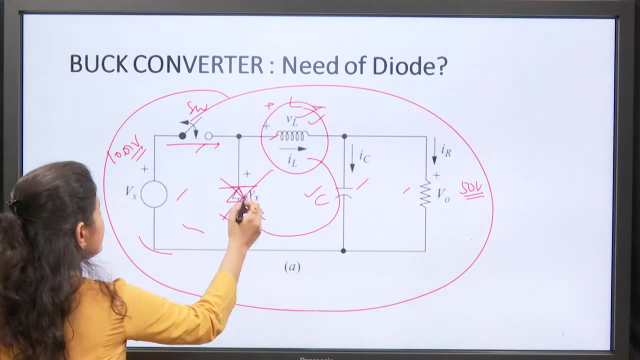 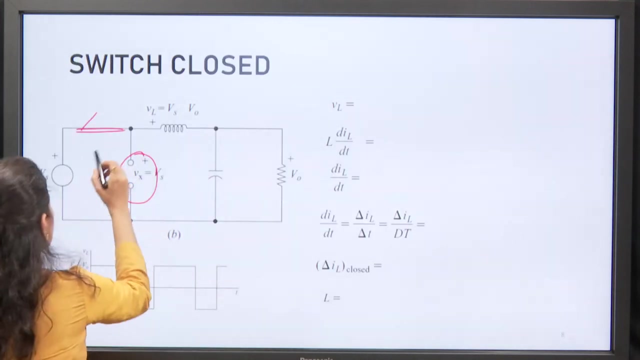 Here. switch was connected when it was closed means when it was conducting. then this diode was connected in the previous circuit. with this current is flowing in this direction. So when switch is closed, current is flowing like this. So there is no need. 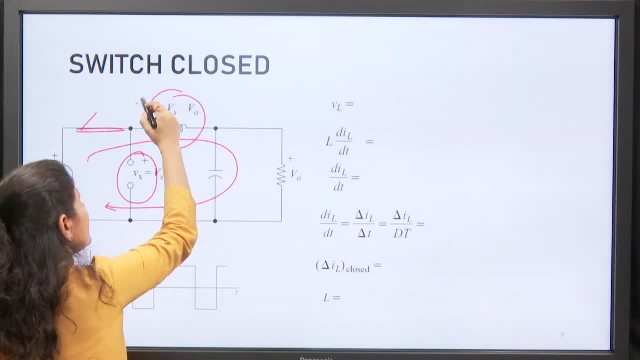 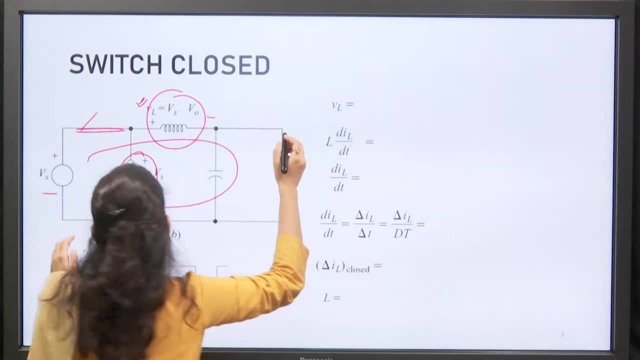 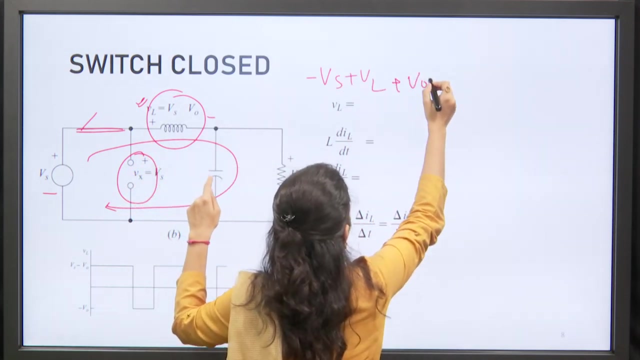 of diode. This cycle is energized. Now, if we want to apply voltage of VL, then apply KVL. from here: This is minus plus, this is plus minus, this is plus minus. So where we are entering minus Vs, then here plus VL. 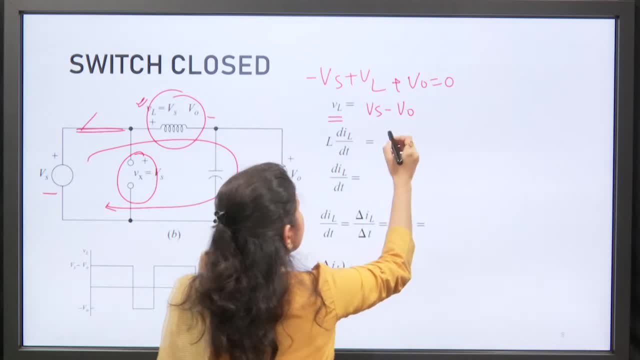 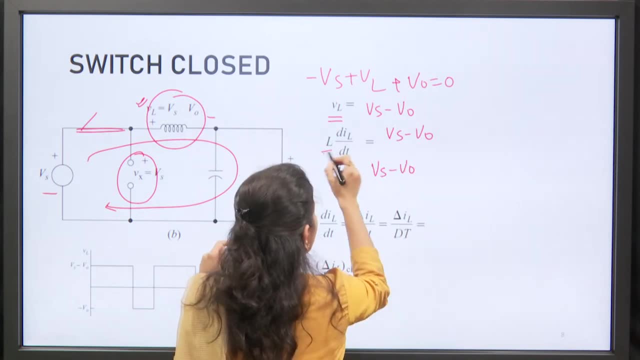 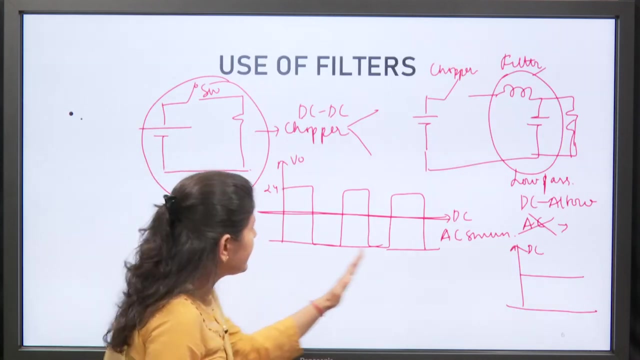 minus V0.. We can write VL L DIL by DT Vs minus V0.. What will be DIL by DT value Vs minus V0, and this L will come in the denominator. Now, one thing which was left earlier is that this output: 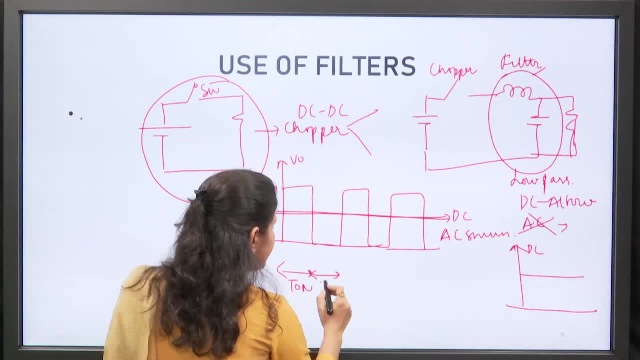 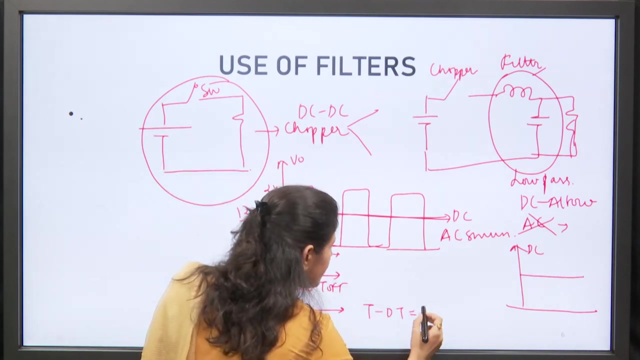 which we were talking about. this output which we were getting this time was T on means DT. This is total time T. We call this DT, So this remaining time is T minus DT. So 1 minus D and T is common. 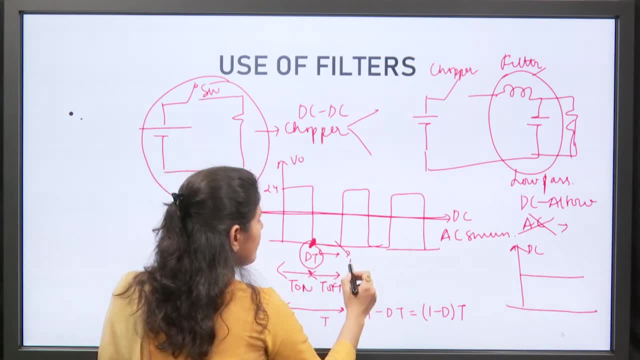 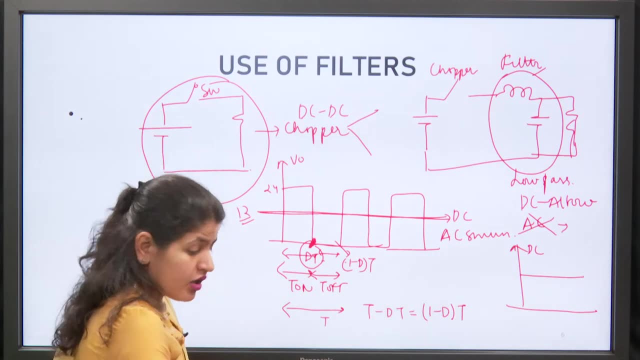 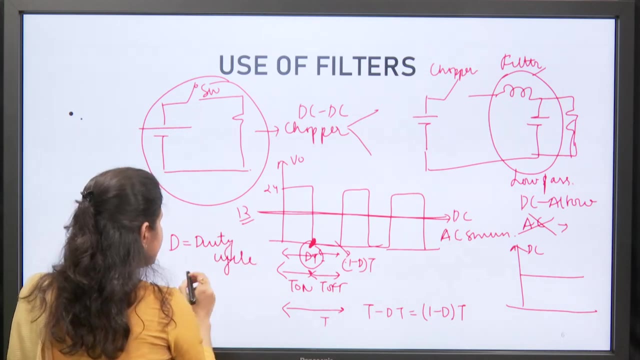 So this time, or this instant is DT and this instant is 1 minus D of T. So this is DT and this instant is 1 minus DT. D is duty cycle which is equal to T on upon T on plus T of means. 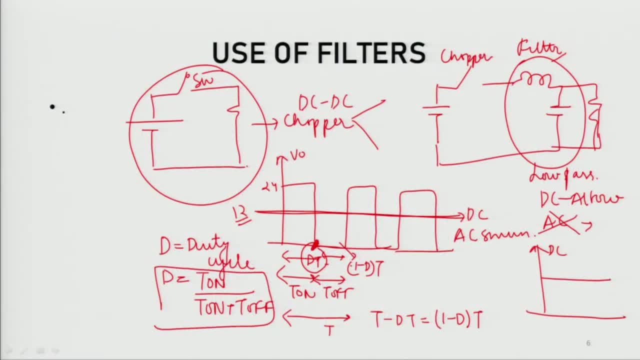 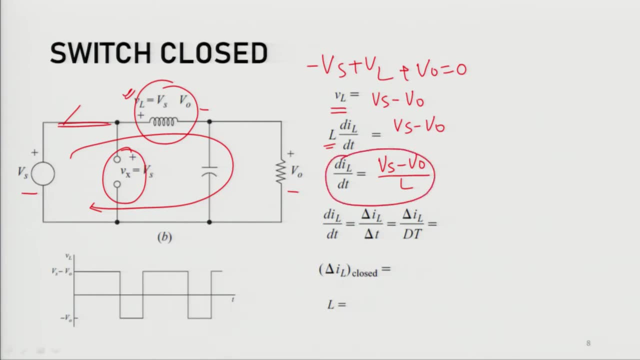 T on upon total time T. This is duty cycle. This is very important parameter. Now, why did I explain this term here? This term, DIL by DT is equals to DEL. IL upon DEL T. Now, this DEL is equal to DEL. 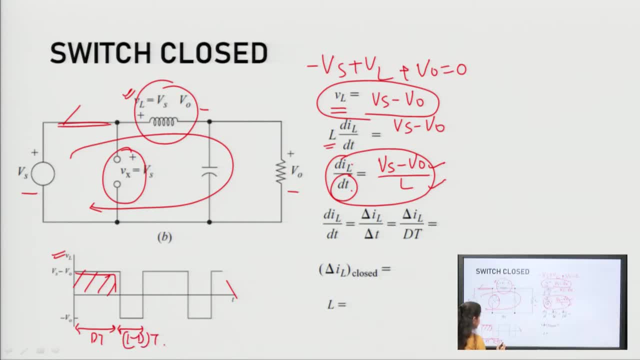 IL upon DEL T. So the time of DEL T is delta t in differential form of close. ki baat kar raha hai yaani, jab circuit conduct kar raha hai, toh wo time hai dt, toh isliye is d t time ko ya delta t. time ko mne d t se replace kar raha hai, toh isko m kya. 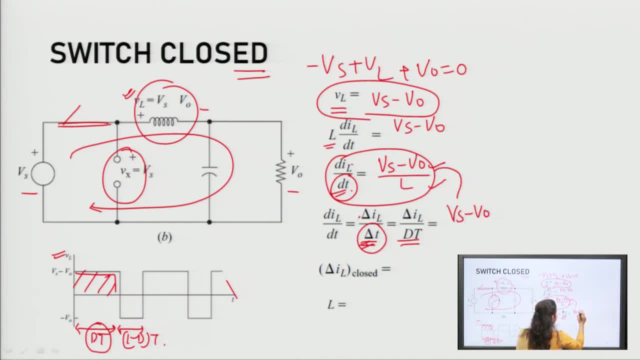 likh sakte hai yahi wala term vs minus v naught upon l di l by dt ko hamne del i l upon d t kar raha hai kyunki ye d t yahan pe ye hai jitna time tak circuit conduct. 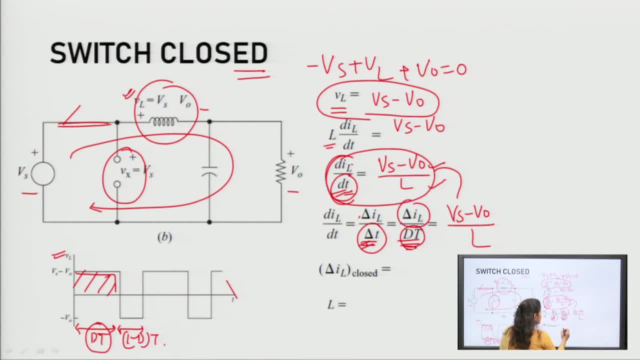 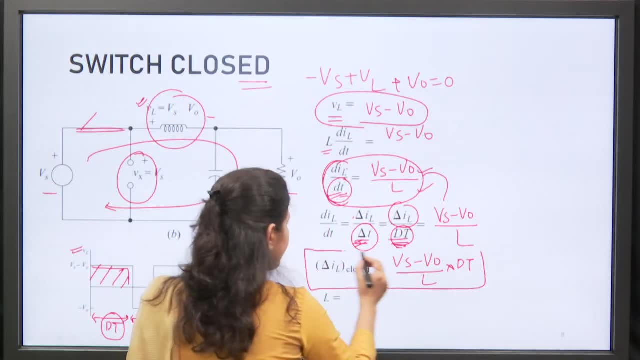 kar raha hai ab yahan se, agar hamme del i l ki value nikalni hai. toh kya kar sakte hai vs minus v naught upon l into dt ye aagayi del i l ki value agar hamme is l ki. 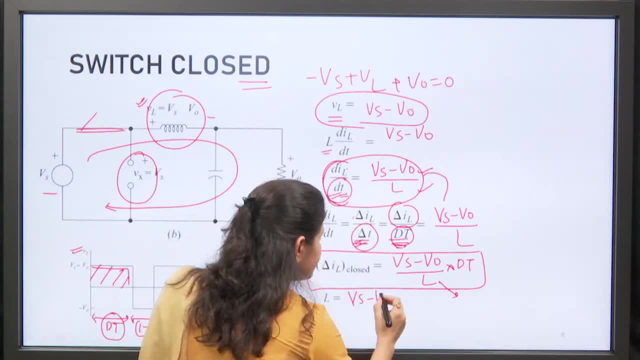 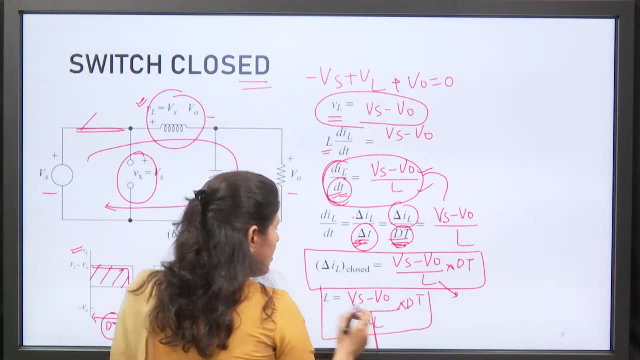 value chahiye. toh kya garengi l upar leke gaye: vs minus v naught upon del i l into dt theek hai, aur ye wala jo t term hai, isko ham ye bhi likh sakte hai: vs minus v naught. 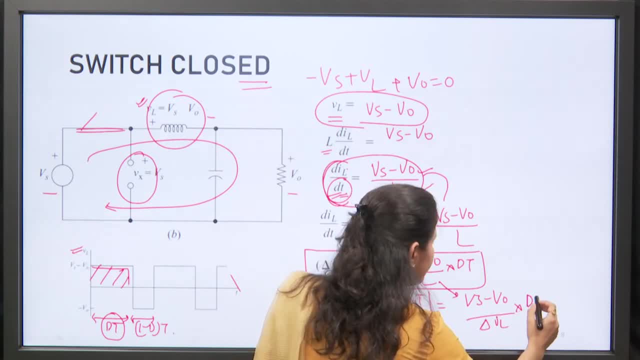 upon del i l into d into time. ko ham kya likh sakte hai. t is equals to 1 upon del i l upon f. hota hai 1 upon frequency yaani into 1 upon f. toh ye aagayi inductor ki value. 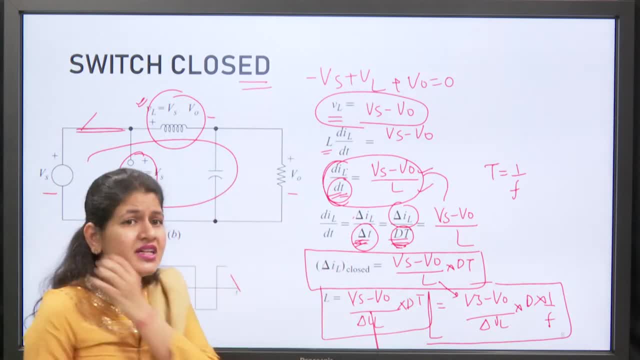 theek hai, ye hai inductor ki value dekhe. toh isse hamme kya bata chal raha hai, is wale term, se hamme ye bata chal raha hai, ki agar kabhi bhi hamme kisi application ke liye 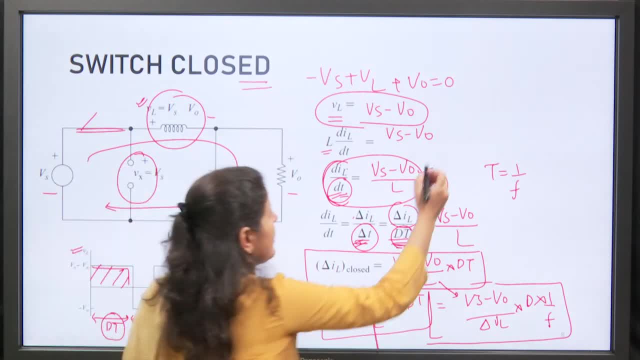 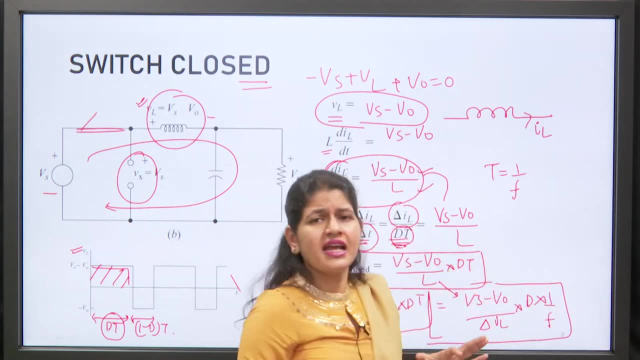 ripple current de rakhi hai del i l kya hota hai? ripple yaani, agar koi inductor hai, us inductor ke across, agar i l current flow kar rahi hai, toh jo generally practical applications me generally jo delta i l hota hai, wo hamme given rehta hai. 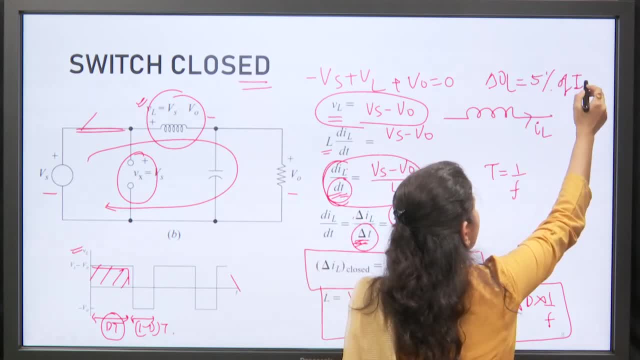 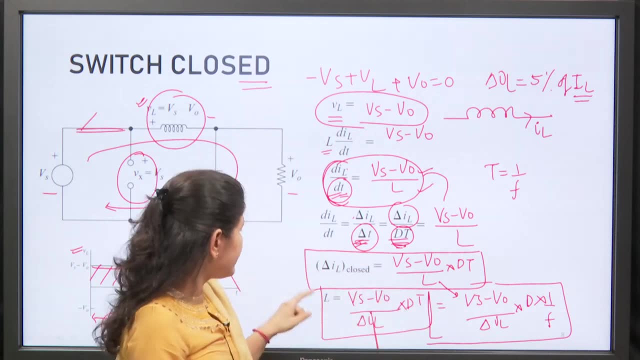 delta i l kahe dete hai, wo ki 5% of i l hoga. theek hai, yaani, jitni bhi inductor current aari hai, uska 5% hoga. toh agar hamme delta i l ki value pata hai, toh delta i l ki value. 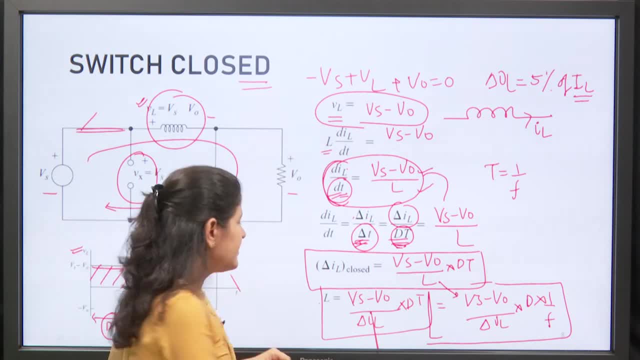 is wale formulae mein yahan pe rakhe: ham inductor ki value nikal sakte. theek hai supply voltage hamme pata rehta hai output hamme pata hai, duty cycle hamme given rahegi. 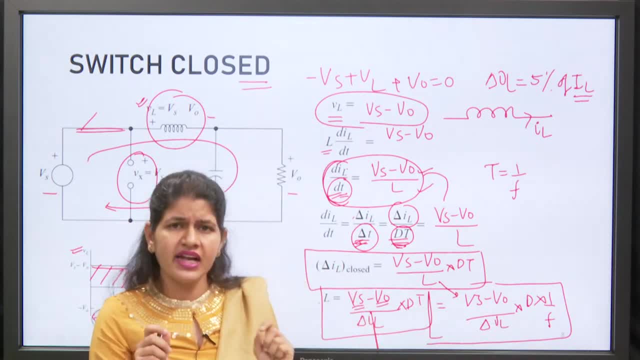 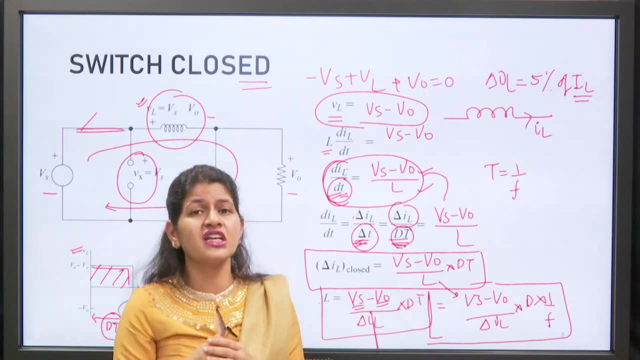 switching frequency hamme given rehti hai switching frequency, ye baat agar aaye switching frequency ki. toh ma ek cheez aur bata de rahi hu, ki ye jitne type ke dc to dc converter hai, ye bohat zyada high switching frequency pe kaam karte hain, high switching frequency se. 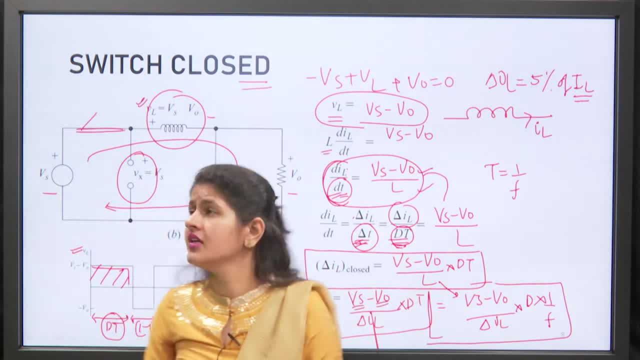 mera kya matlab hai. mega hertz wali switching frequency me kaam karte hain, toh yaani yahan pe ye jo switch use kiya jata hai. ye aise switches hote hain, mosfet type ke jimki switching. 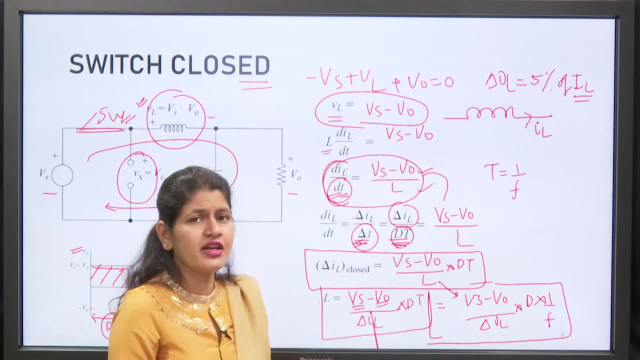 frequency bohat zyada high hoti hai. uska advantage kya hai? wo aapko yahi dekhne ko milega, agar ye frequency bohat zyada high ragde, toh kya aur raha hai ye frequency? 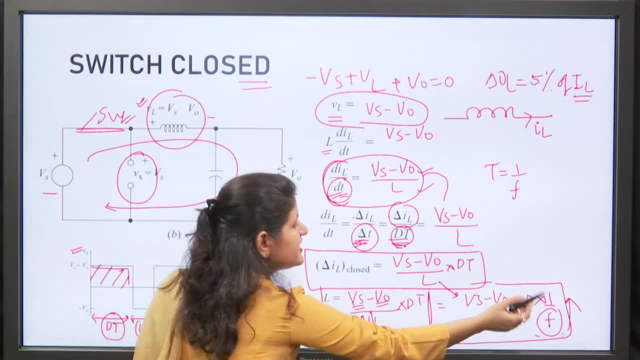 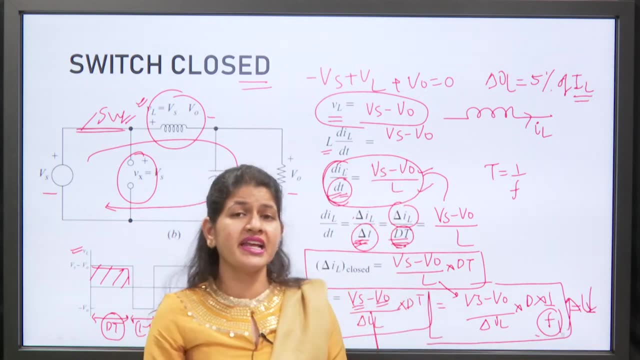 is inductor ke inversely proportional hai. hai na ye frequency agar this is equal to l. hai Ye frequency agar bohat zyada high ragde, toh inductor ki value kaam rakni padegi, aur abhi humne pehle ye baat ki bhi hai, ki inductor apne aapme bohat bulky element hota hai, toh 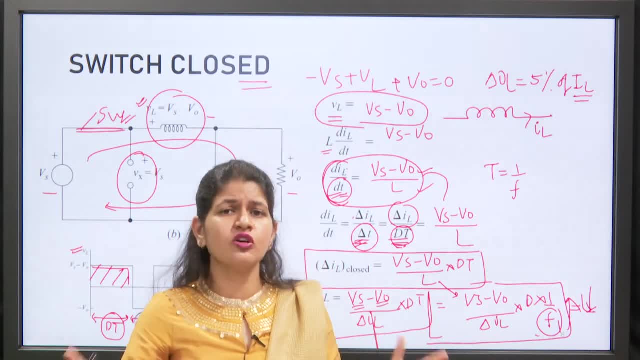 jitna bada inductor lagayenge, utna zyada cost hoga, utna zyada complex hoga circuit theek hai. toh aise bohat sare disadvantage hongi jiski wajah se hum ye switching frequency. 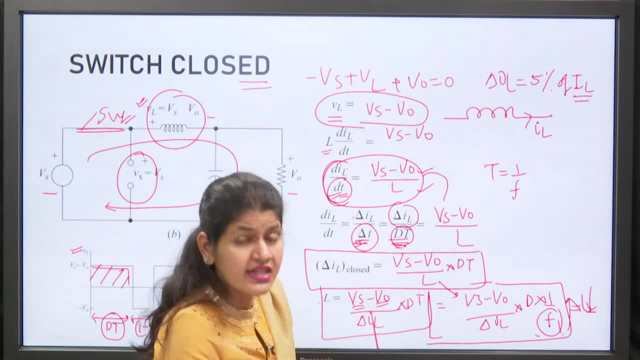 high rakte, taaki inductor ki value hume kaam rakni pade Theek hai. iske disadvantage bhi hai: frequency zyada switching, frequency high rakne ke disadvantage bhi hai, ki usme power loss zyada hota hai. 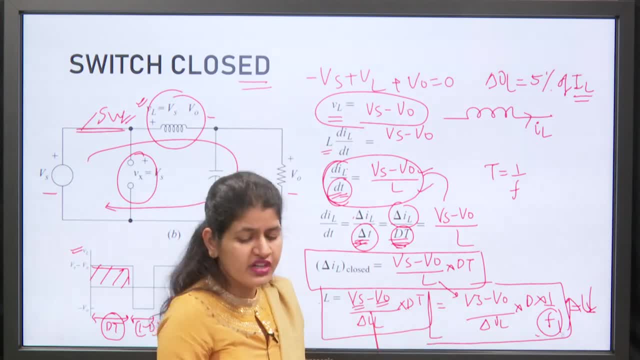 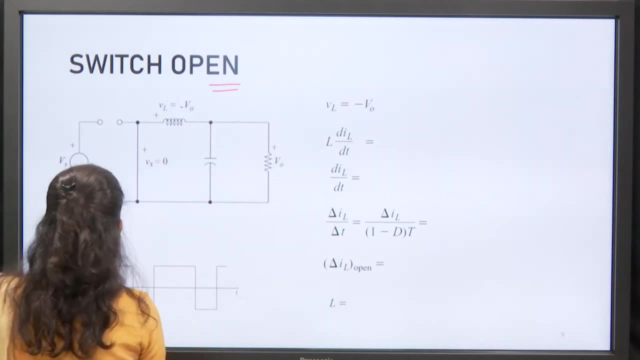 Theek hai, toh trade off karke, hum ye switching frequency rakte hai. theek hai, ab switch open? dekh liye, jab switch open hai, toh kya ho raha hai? bilkul same process hum follow karenge. 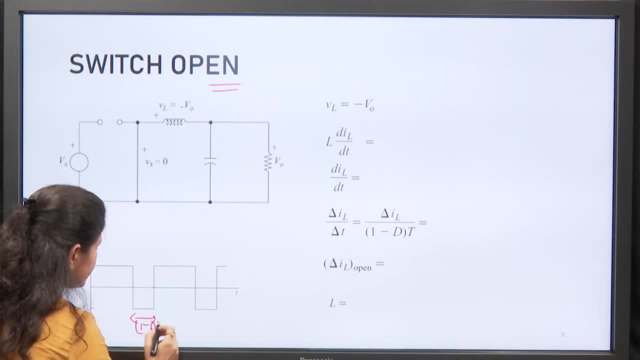 open hai toh yaani ye wala time 1 minus dt theek hai ye wala time hai toh VL is equals to minus V. naught hai na kyunki tab ye diode conduct karne, lagayega ye jo inductor hai. 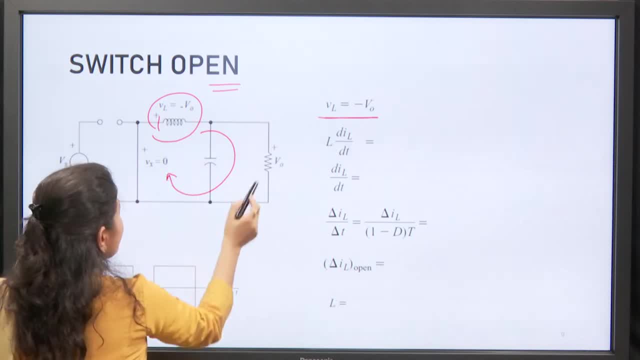 bo is diode ke through apne energy release karega, toh iske andar. agar lagayee KVL, toh VL is equals to minus V. naught aayega l by dt. kya ho jayega l by dt, kya ho jayega l by? 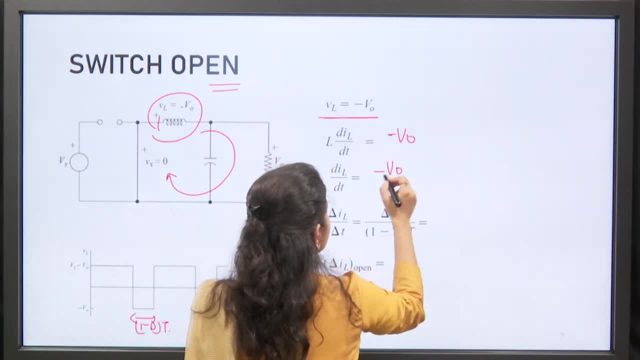 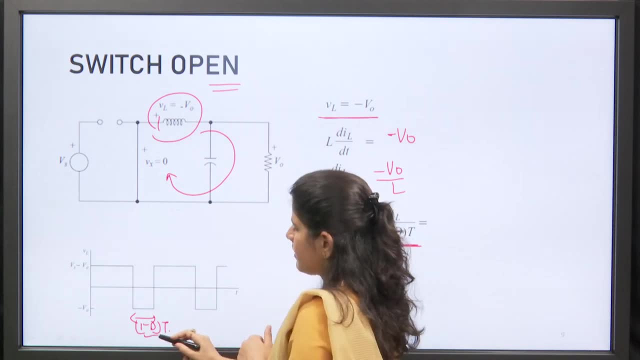 dt kya ho jayega minus V naught, wave jayega minus V naught upon l aur yaha pe jo ye dt wala time hai, ya delta t wala time hai, wo ho jayega 1 minus d t theek hai 1 minus d. 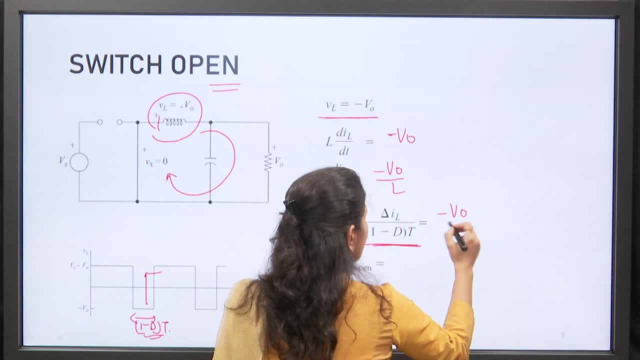 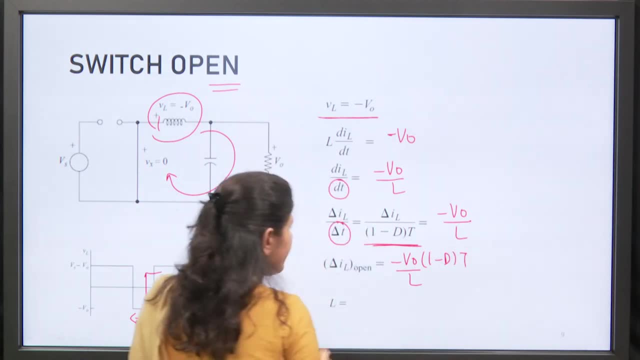 t kyunki yahi off time hai theek hai toh. is ki value. kya ho jayegi minus V naught upon l, aur ye ho jayega minus V naught upon l 1 minus D of t theek hai toh ab. 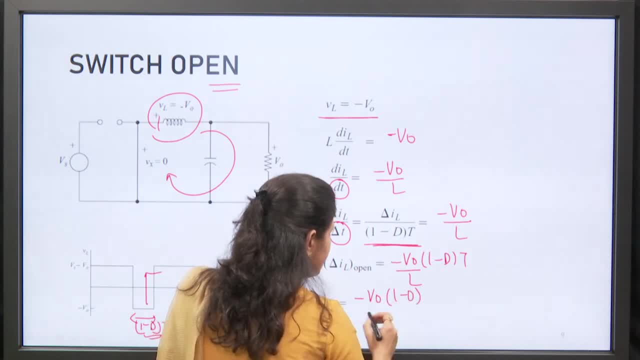 l ki value. kya ho jayegi l agar idhar le aaye. toh minus V naught one minus D upon delta i L L by dt V0.. l by dt 1 minus D, and this t term we can call as 1 upon f frequency. 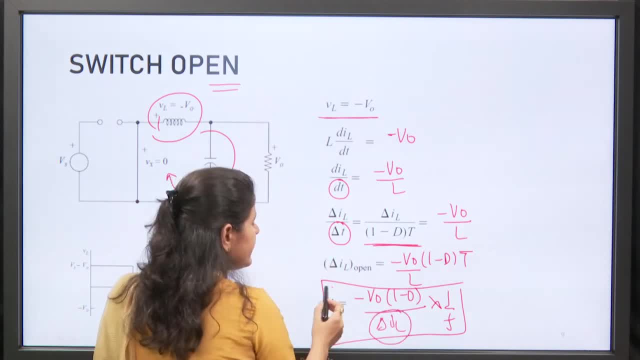 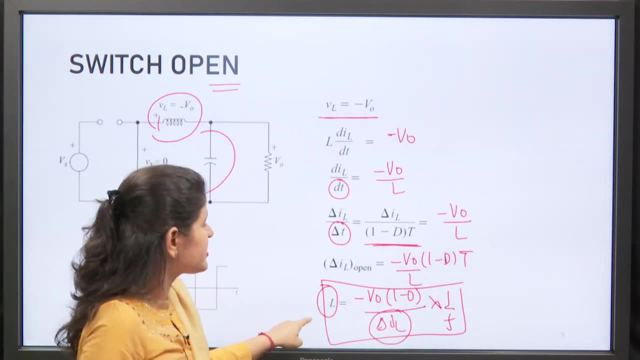 So see here also: if we get the value of delta iL, then we can get the value of L. So whether it is switch on circuit or switch off circuit, you are getting two expressions of L in both of them, So you can get the value of inductor from any expression of both of them. 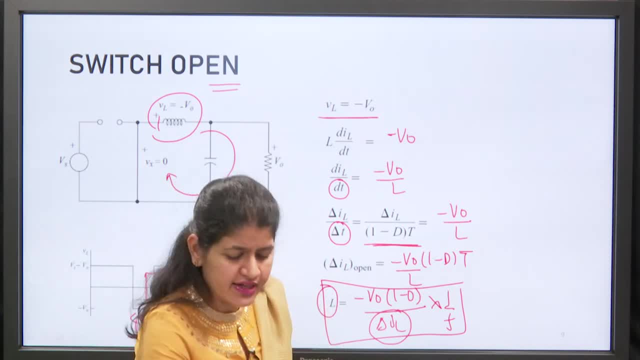 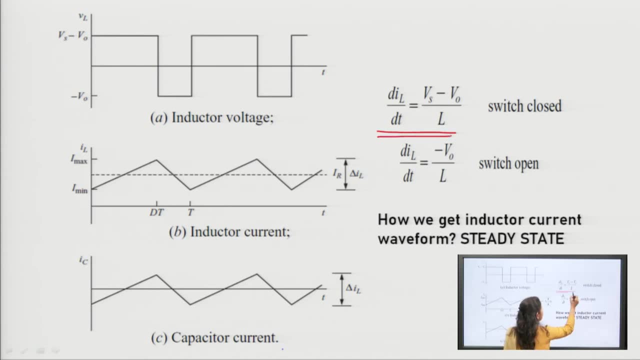 whichever you want to use appropriately, So you will get the same value from both of them. So see, this kind of inductor, current waveform is coming. We have taken out these expressions: DIL by DT, DIL by DT When switch is closed and when switch is open. 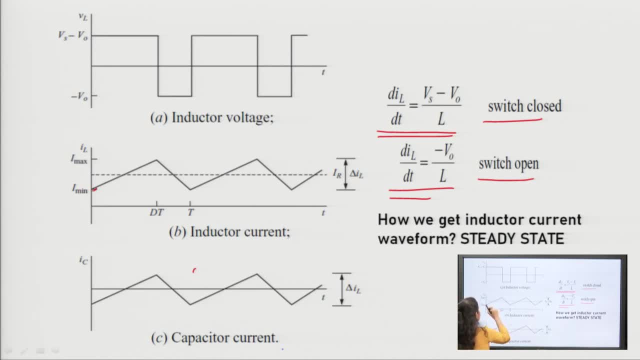 from here. we just want to see how the waveform of inductor is getting In. this time, DIL by DT has a positive slope, So see, inductor is getting energized and in the next time, this negative slope- inductor is getting de-energized. 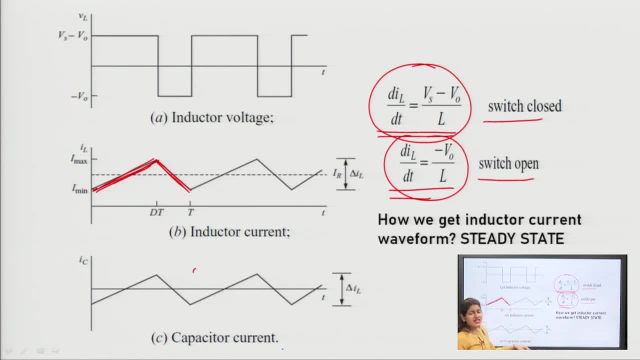 So one more thing we get to know is that the value we have given inductor's waveform is a steady state waveform. When inductor is charged for the first time, it will start from here, from zero. Then it will be energized. 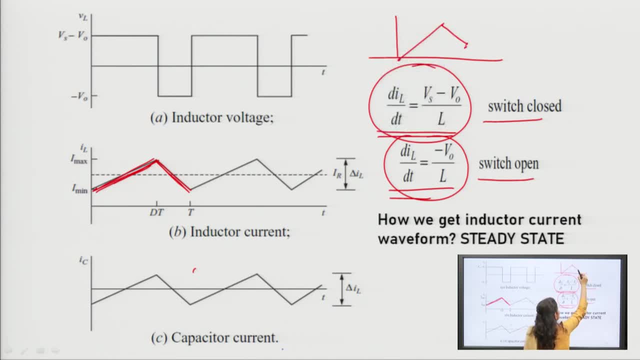 then it will be de-energized here. then it was de-energized till here. till then it will be energized again. So we have given steady state value. Steady state means after some time, when it will reach steady state value. 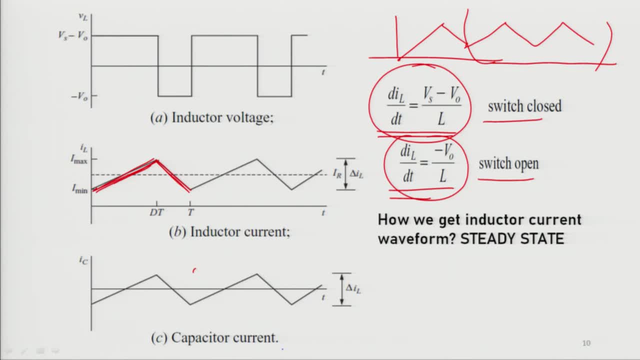 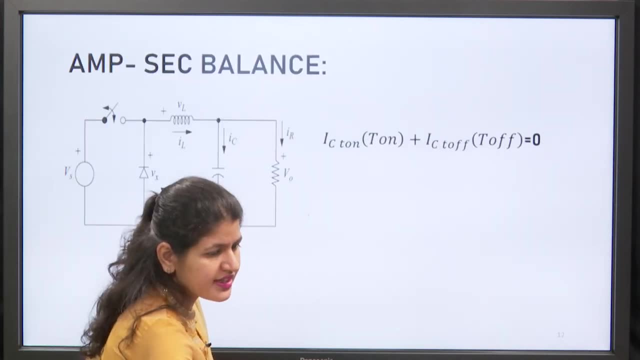 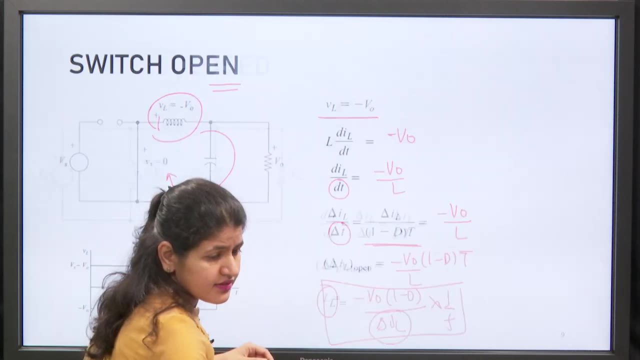 we have given its value, Its initial value will be from zero. only Now see IC current. The waveform of IC current is also the same. You can see from here. only This is the circuit. This is the circuit. Let us see from this circuit. 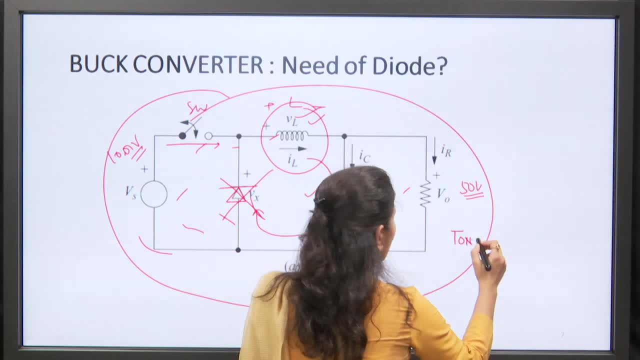 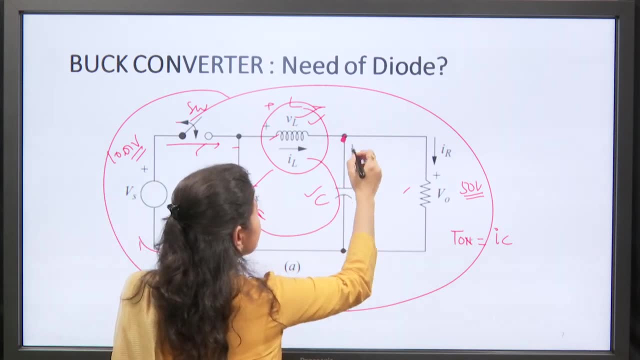 What is visible in this circuit? When T is on means when switch is on, then what is the value of IC? When switch is on, then what is coming Here? put KCL, This IC is equal to IN, which is coming from here. 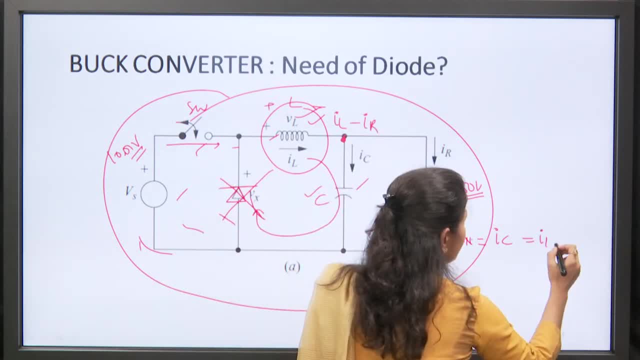 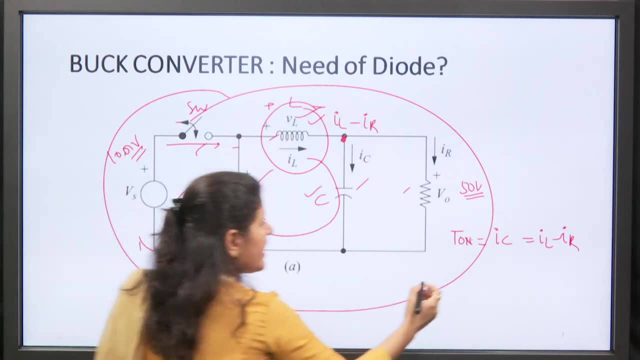 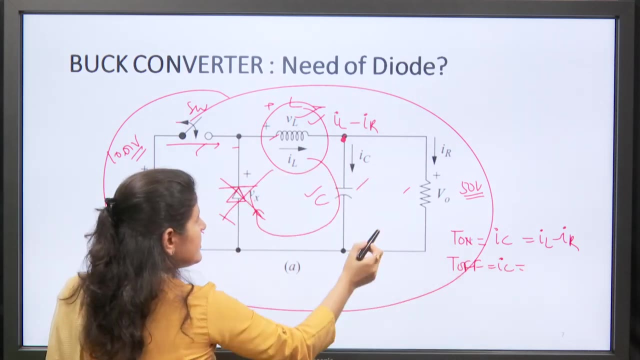 which is IR. So this is IC is equal to IL minus IR. Similarly, when switch is off and current is flowing in this direction, then also IC current is coming. means when T is off, then also IC value is coming. See, current is flowing in this way. 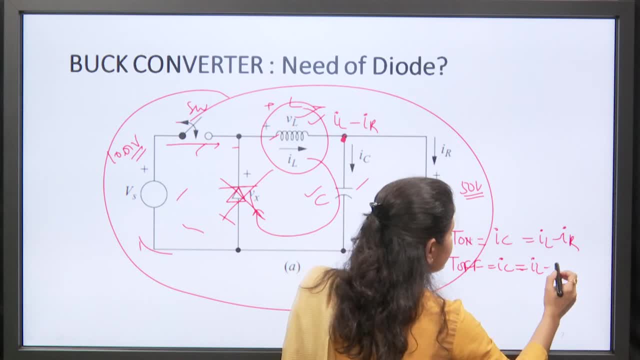 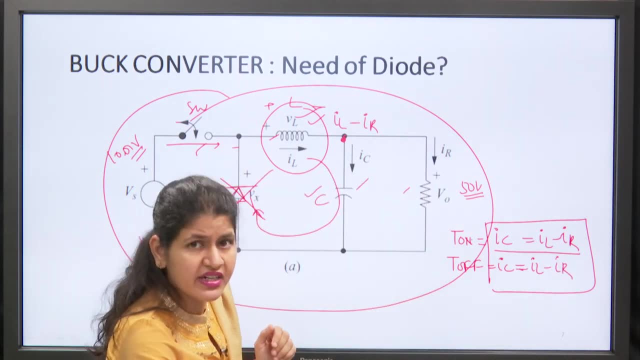 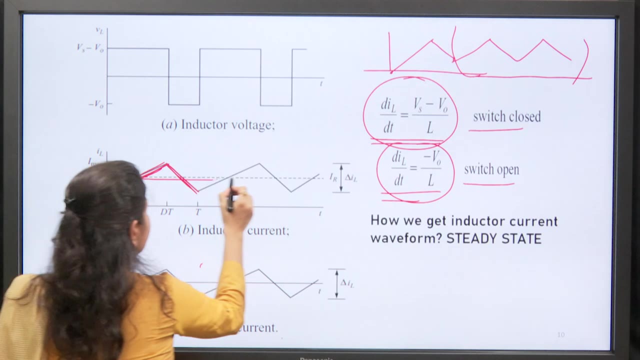 Half is going here, half is coming through IC. Then also, IC value is IL minus IR. So these are the values of IC As we will see in next lecture in more detail. For now you can see in waveform: This is the value of IR. 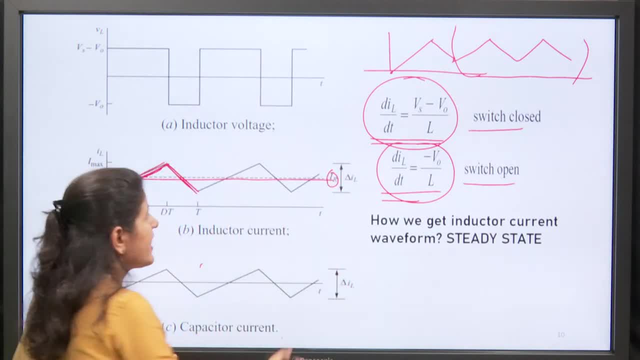 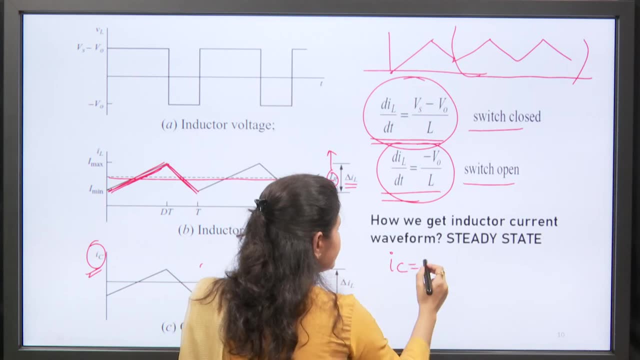 This is the value of IR. In next lecture we will see how this IR is being calculated. This is IR and this is IL, And what we have taken out at the back, IC is equal to IL minus IR, Whether T is on or T is off. 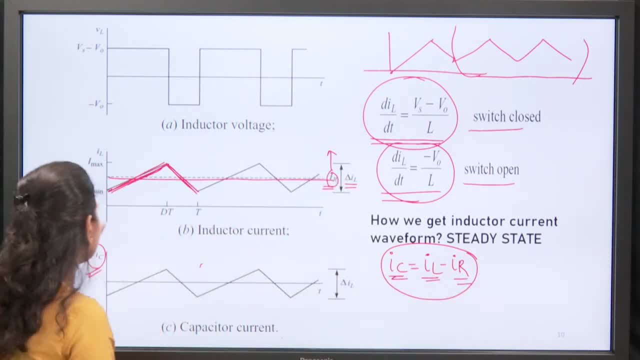 IC is equal to IL minus IR. So let us see from this terminal: This is instantaneous value of IL And this is the value of IR. So from this IC, IL, if we subtract this IR, then it will be negative. 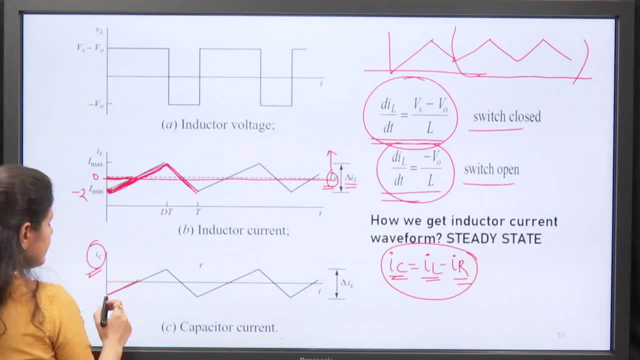 Let us assume this is minus 2 and this value is 0. So this will be negative value. So from this, this waveform is IL and this waveform is IR And this waveform is IL and this waveform is IR. By subtracting these, 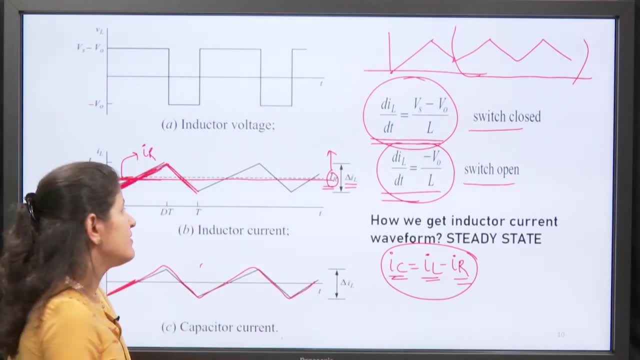 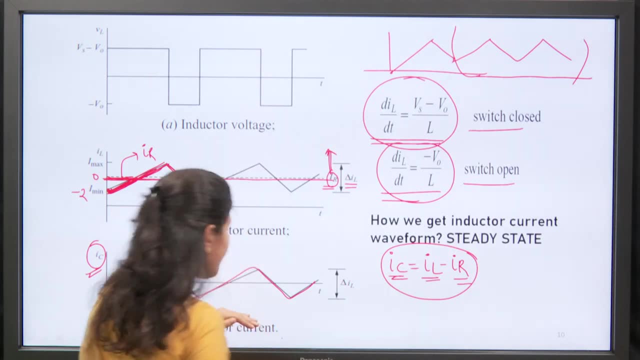 we have got this waveform of IC, So now we will see further how we are getting the value of IR. What is the value of IR Now we will see in next slide, Because here the waveform of IC has come. So you see the waveform of IC. 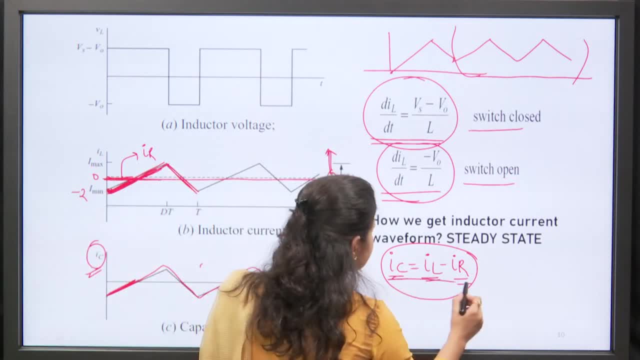 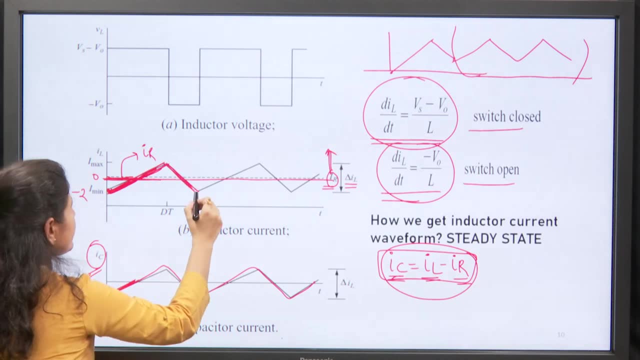 From the previous main circuit we have derived that IC is equal to IL minus IR. So this is the waveform of IC In this. this is IL. This waveform is the waveform of IL. These are instantaneous values of IL And this middle dashed line is IR. 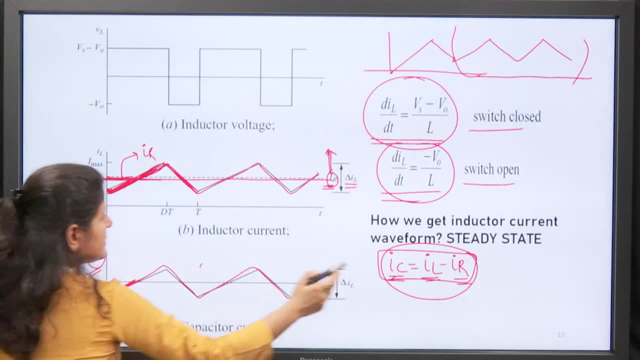 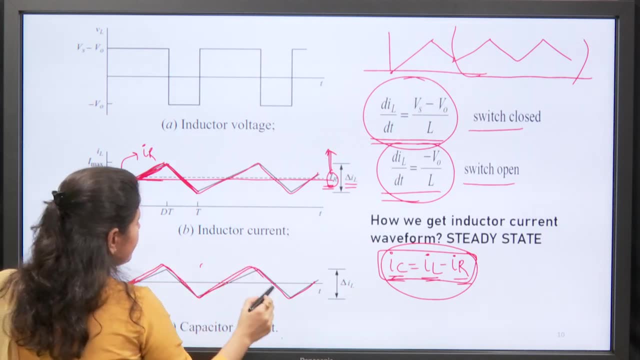 This is the average value. So IC is equal to IL minus IR. This is IL And in this we will subtract the waveform of IR, So we will get this kind of current waveform. Ok, We will see this capacitor waveform in more detail. 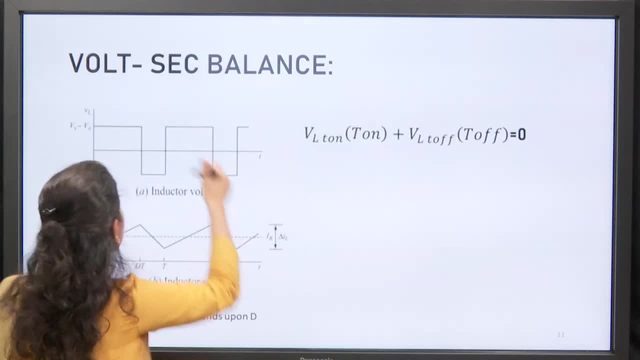 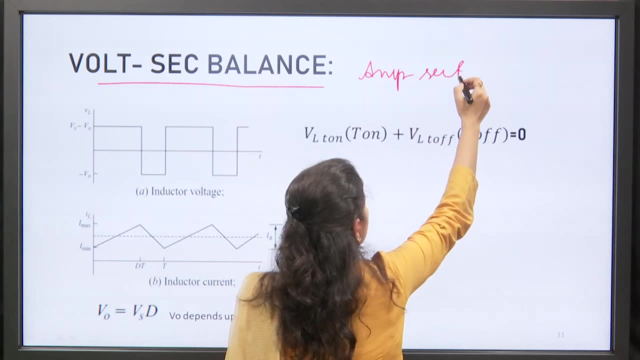 Next, there are two more topics which we will do further in detail. One is voltage, second balance, And after this one more term will come. That will be ampere, second balance. Ok, So first of all know that if we start any analysis,